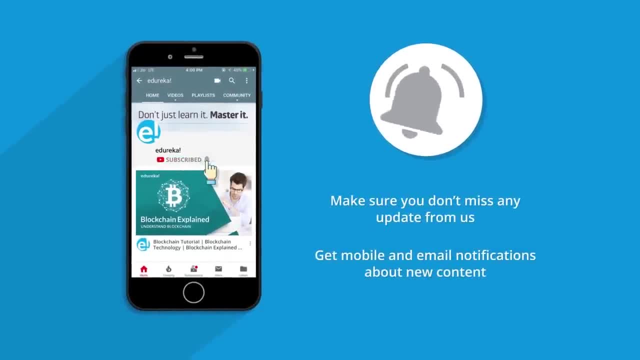 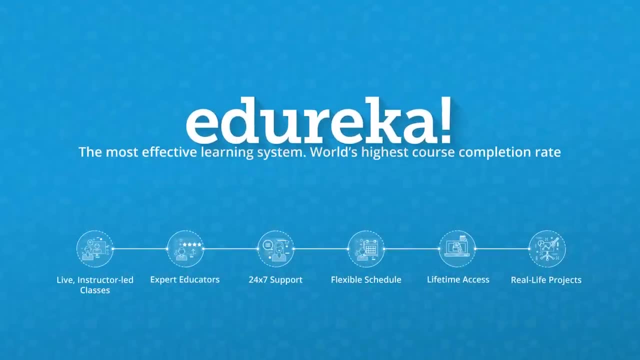 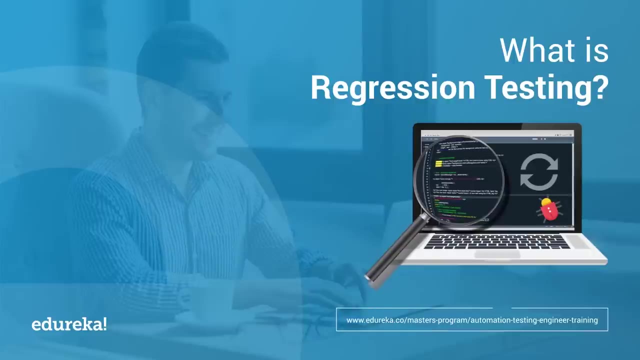 You've all been there. You make a tiny change in your code and suddenly another part of your code stops working. You're just hours away from an important release and panic sets in. How can changing that one variable cause everything to fall over? But then a colleague of yours remembers. 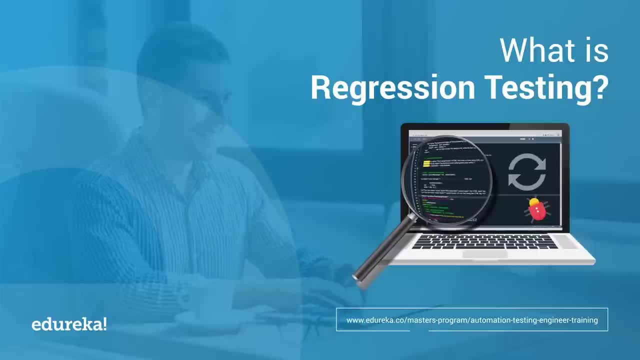 an obscure bug from months ago. Can this be the same thing? This is where regression testing comes into picture. Hey guys, I'm Archana from Edureka and I welcome you all to this session on regression testing. But before we proceed, let's take a look at the topics which we will be talking about today. 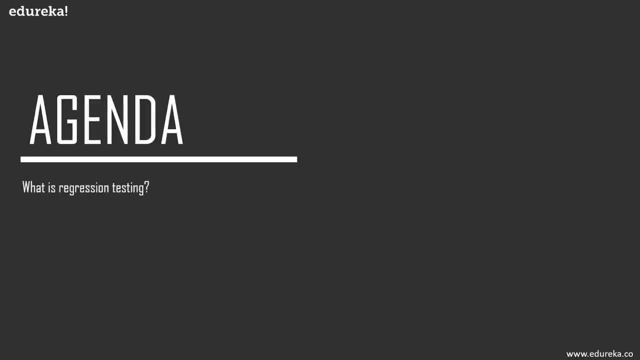 So we will begin this session by discussing what is regression testing and benefits of using regression testing. Moving on, we'll see when to apply regression testing. Then we will check out types of regression testing, how to do regression testing and techniques of regression testing. 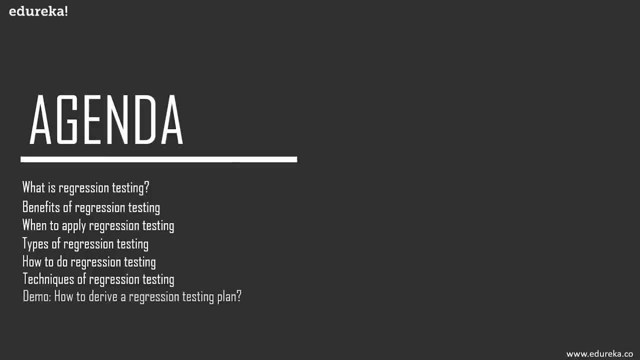 and then comes the interesting part: We'll be doing a demo in which we will see how to derive a regression testing plan And finally, we will end this session by talking about regression testing challenges and best practices that you should follow while performing regression testing. 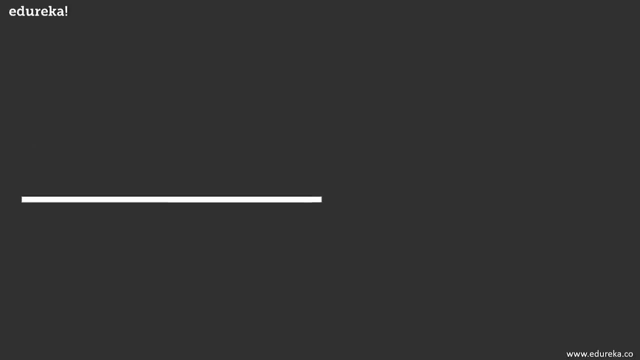 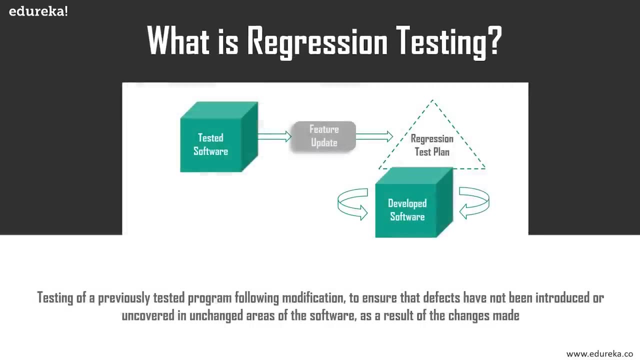 So I hope agenda was clear to you guys. Let's get started there. So what is regression testing? A regression test is a system-wide test that's intended to ensure that a small change in one part of the system does not break existing functionality elsewhere in the system. It's. 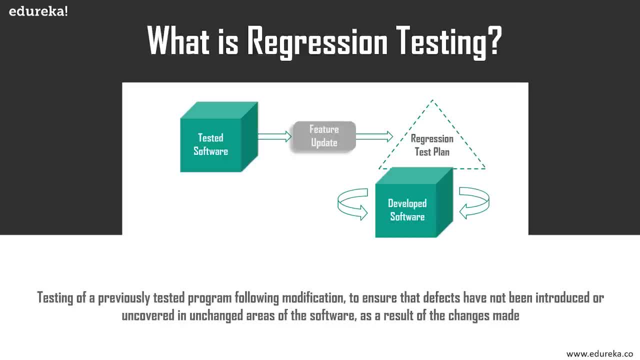 important because without regression testing, it's quite possible to introduce intended fixes into a system that could create more problems than the solves. So let me give you a simple real-world example. You take your car to a mechanic to get the air conditioning fixed, and when you get it back, the air conditioning is working. 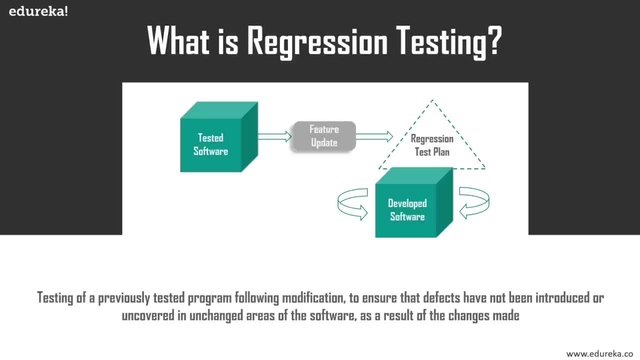 Properly, but the gas tank sensor is no longer working. If regression test is an unintended change, then regression testing is the process of hunting for those changes. Put simply, regression testing is all about making sure old bugs don't come back to haunt you. Let's take a look at 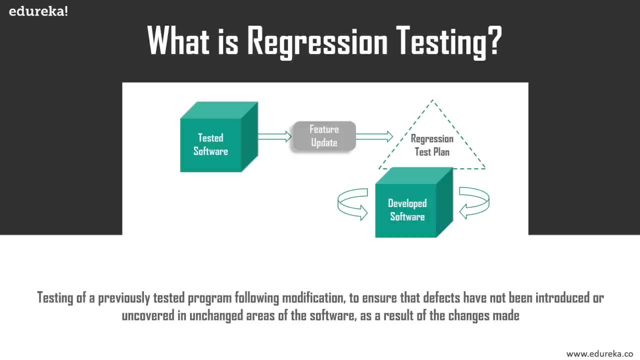 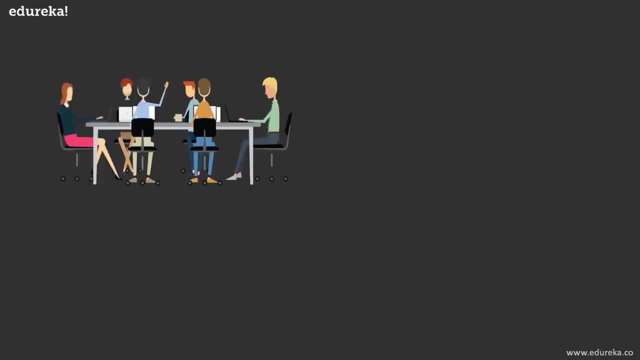 technical example that illustrates what can happen when regression testing is not used. So one day the manager of accounts receivable department at Wayne Industries uncovered a bug in companies financial system. It turns out that the module responsible for reporting overdue invoices was not listing all the overdue invoices. The bug was assigned to a developer. 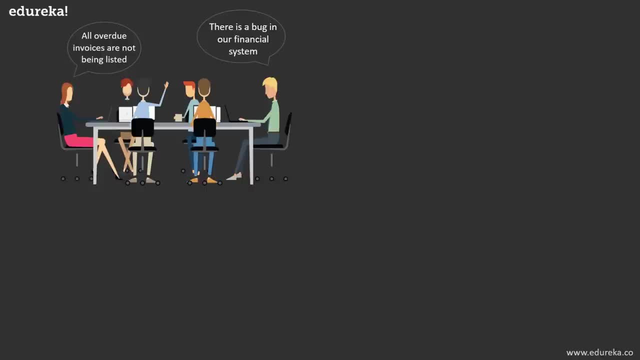 to make the fix. the developer followed company policy and unit tested the new code. the unit test proof beyond a shadow of doubt. that fix worked as intended. developer did a good job. The fix was released into production. so far, so good. a week passes, then a strange behavior. 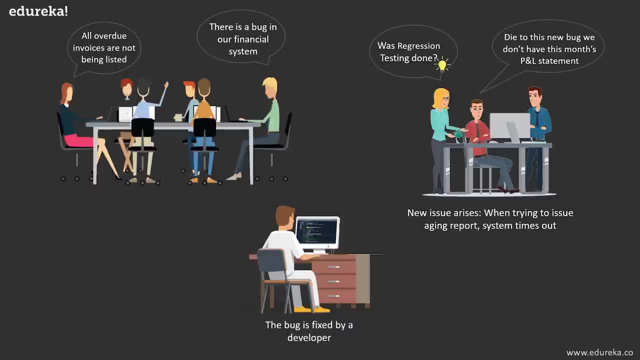 occurs, Accounting Department tries to run the company's month and profit and loss statement. whenever the system tries to issue an aging report, the system times out. So what is aging report now? aging report separates and sums invoice amounts according to age, like 30 days past. 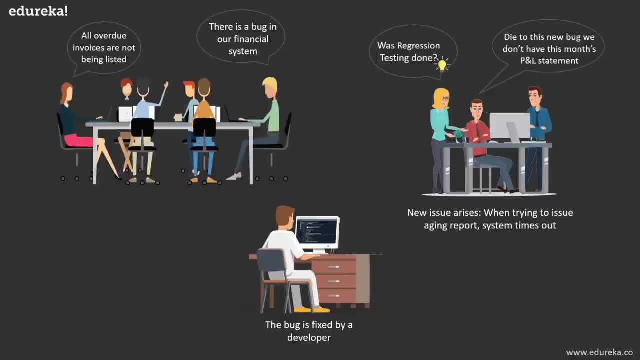 you 60 days past you, 90 days past you, Etc. So what happened was when they were trying to issue an aging report, the system timed out without its month and profit in late statement. The company doesn't know if it's making money or losing money. The accounting department is really upset about. 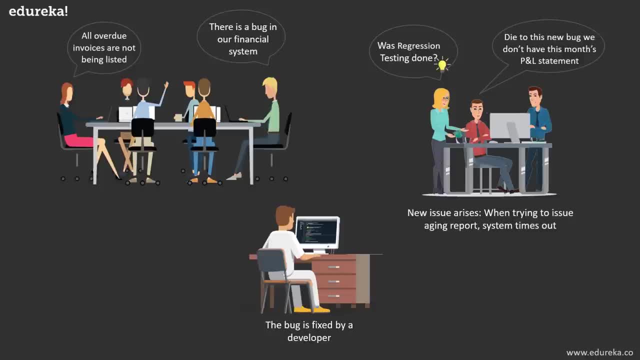 it, The accounting manager contacts the software development manager to report the issue and seek remedy as soon as possible. So tech leads and quality analyst manager brought in to find out the issue. turns out that the new code which was encapsulated in the function was only tested for small database when the same was applied for production data, which 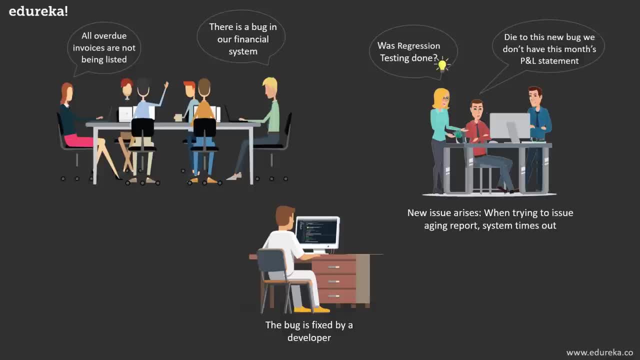 is usually very large. the code didn't work as expected, So what you have to notice here is that If the fix had been incorporated into system-wide regression test that used a copy of data running in production, the chances are very good that issued have been resolved before the release. 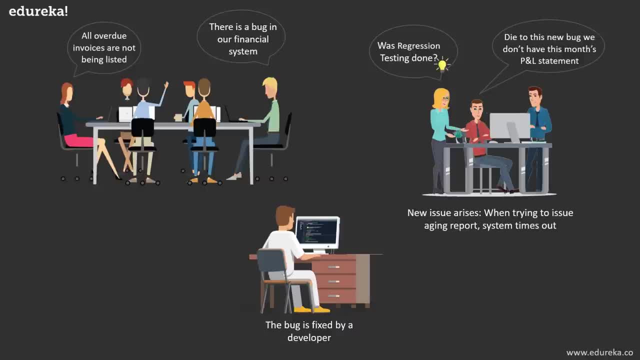 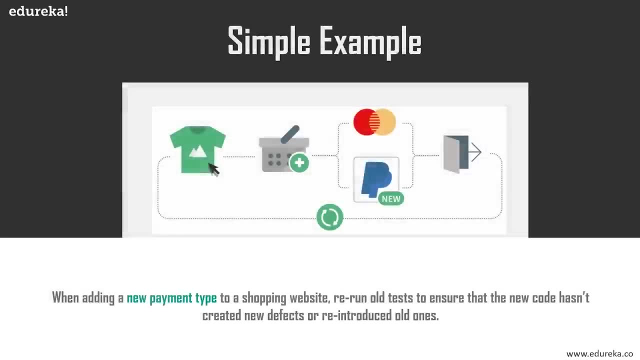 to production or discovered. actually, that's how important regression testing is. Well, that was a little technical, right. Here's a simple one. This is just the testing of a simple e-commerce website, and here we're checking the functionality of payment options. So first, 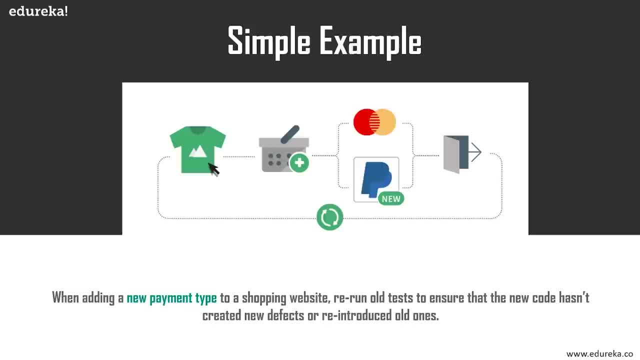 of all, there was only one payment option, Let's say credit card. So item has been added into card. You use the one payment option which is available, then make the payment and everything is working properly when tested. now the company wants to add one more payment option, Let's say PayPal. So now the company checks. 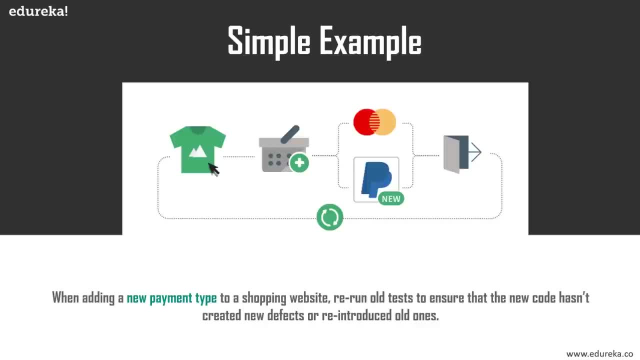 if the option of using PayPal is working properly or not. So again, the item is added to card, The payment is made through the new option which is added, and everything is working again. Now what company does is? it goes ahead and test for the previous payment option again. 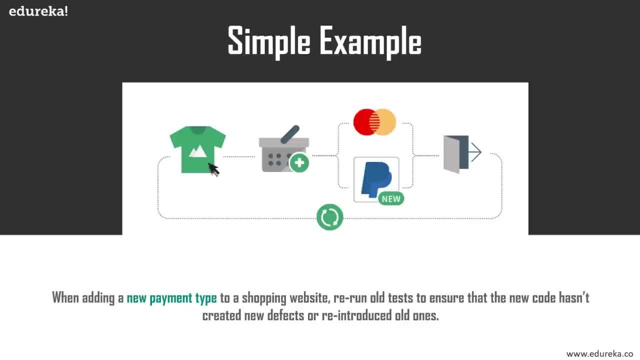 then they find out that the previous payment option is not working properly. So what happened here? the new payment option, which is PayPal, has affected the old one, which is credit card. So what they do, the perform regression testing. So what they have done here is they've checking if the new payment option has affected the old one. 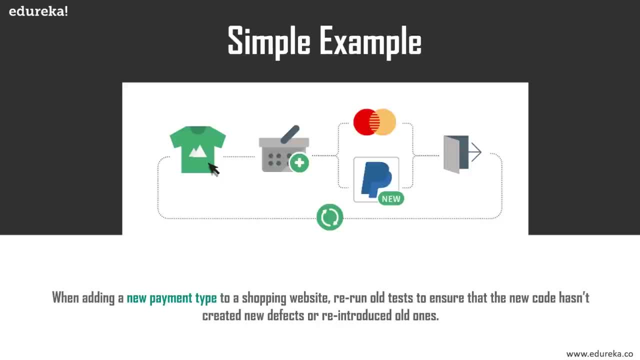 in any way. if so, the box are identified and resolved. that's what regression testing is all about. So, basically, this regression testing is not just done at the beginning, It's done throughout The the testing phase, and that we call regression testing cycle. 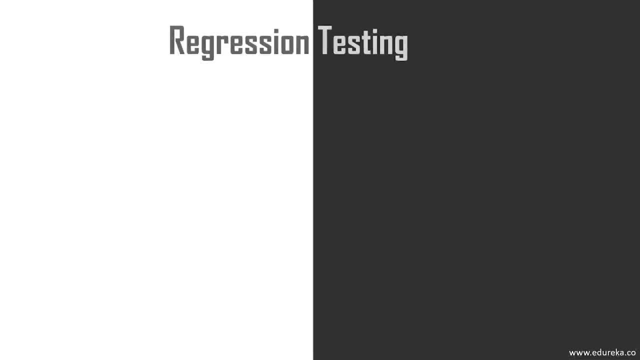 Let me show it to you guys here. it is So as you can see, the one on the left side is the regression cycle. So you incorporate your cold into the bill and schedule the test is you find a bug, resolve it and write your regression test again based on those bugs. 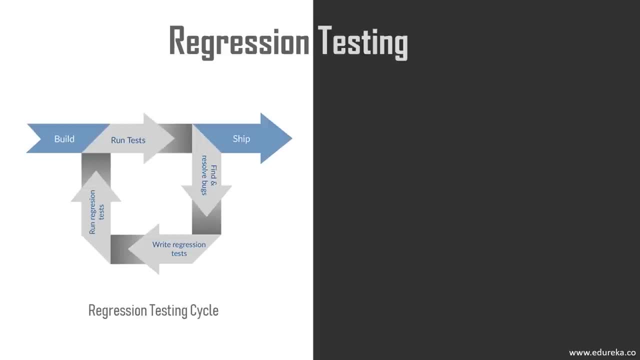 and the fixed issues and run those regression test and the cycle goes on until you get a perfect product and then you release your product into the market. So that's what we call a regression cycle, And on the right side you have a graph which represents what regression testing is basically. 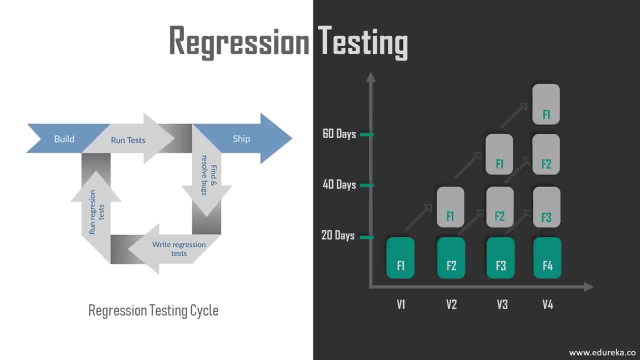 let's say you have version one of your any software product and this is the feature one which you have enabled during the version one and that was released after 20 days of its development. and then you have version two or release to you have added new feature F2.. 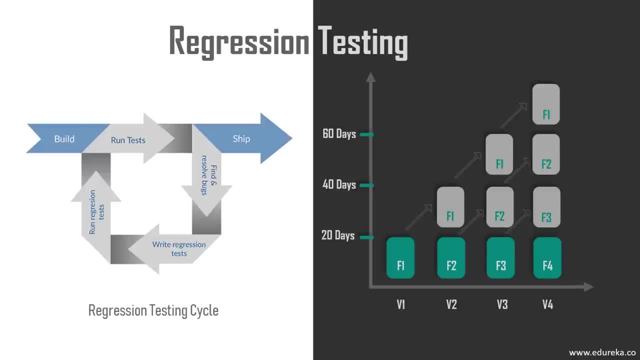 It's working properly. So you go ahead and check if F2 has affected F1 in any way. That's what regression testing is all about. and your second release is released after 40 days. Similarly it goes on. next version: you add new feature, you check out. 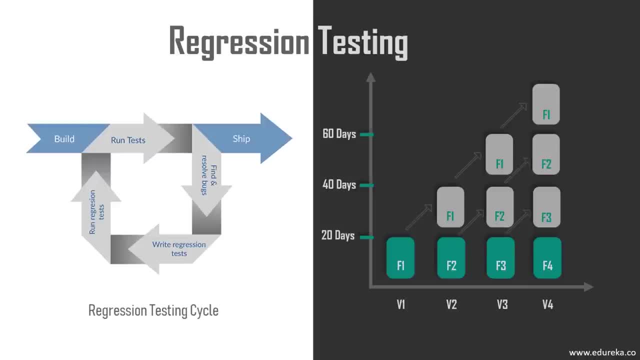 if the other features or the previous features are dependent on it, If there are any errors because of the new feature. if no, then you release your product. So that's what regression testing is. So I hope, after so much explanation, you guys are clear. 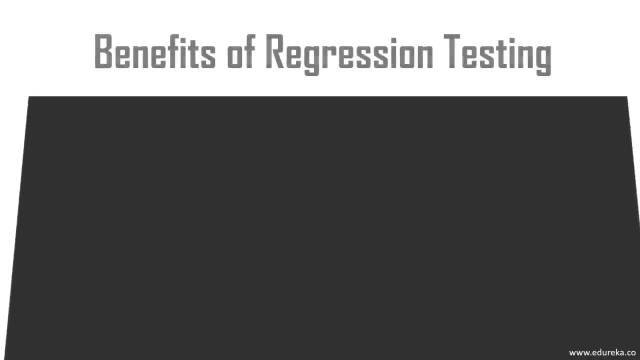 with what regression testing is right. Yes, let's carry on that. Well, the basic aim behind conducting regression testing is to identify box that might have got developed. you to change this introduced. Conducting this test benefits in number of ways, such as: the regression testing increases our chances. 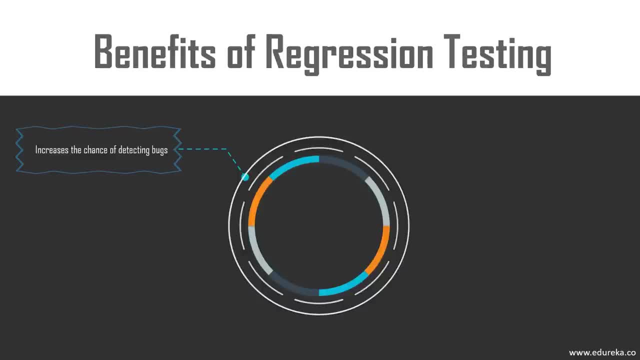 of detecting bugs caused by changes to any software or application. this changes can be anything. It could be just updates or patch fixes or defect fixes or anything during unit and integration testing. regression testing can help catch defects early and thus the reduce the cost to resolve them. 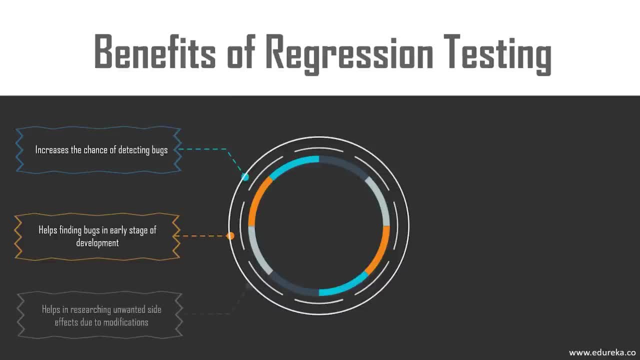 So basically it's cost-effective. it also helps in researching unwanted side effects that might have been occurred due to new operating environment. It ensures better performance software. And why is that? because using regression testing, we can identify box and errors in the early stage itself. because of that, the performance your product is literally high. 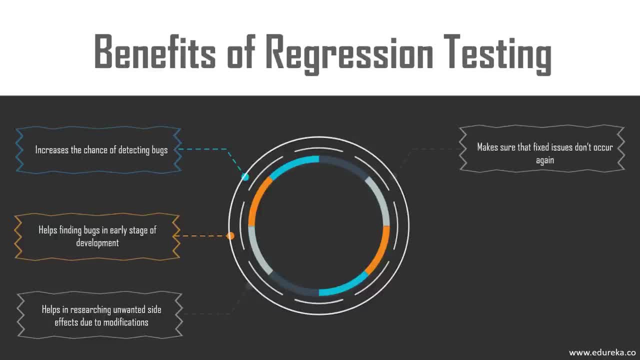 it makes sure that the issues which are already fixed do not occur again. That's one of the best thing about regression testing. Most importantly, regression testing verifies the code. changes do not introduce any old effects, improve the quality of deployed software. this way, It ensures the correctness of the program and, as a result, 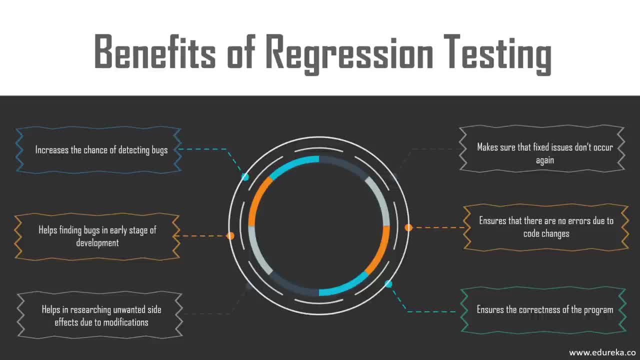 the best version of your product is released to market. So, to summarize, it reduces the amount that you have to pay on your testing. by reducing the amount of bucks and making sure that the old box don't written, it gives you the best product or the quality of product is improved. 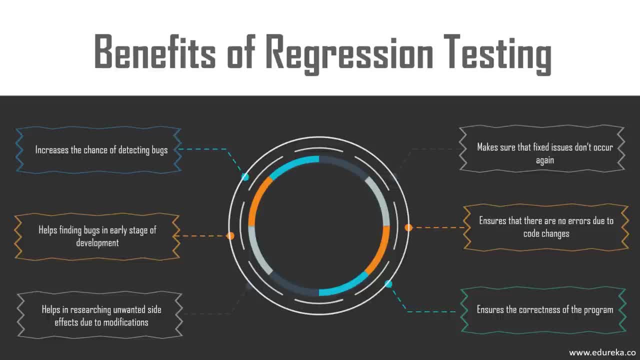 when regression testing is performed and you can actually catch the box or any kind of issues in the early stages itself. So these are some benefits of regression testing. However, in real world, designing and maintaining a near and finite set of regression test is not actually feasible. 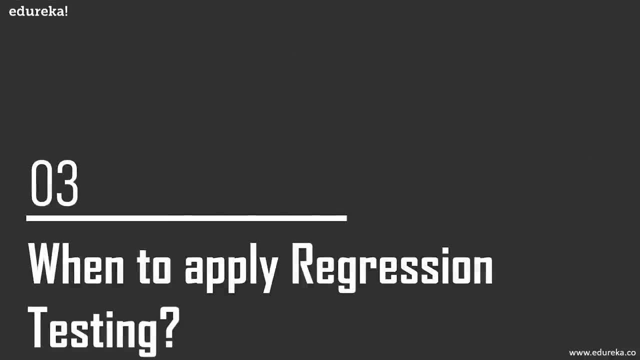 So it is important to determine when to perform regression testing and when not to regression test of frequently executed throughout the software testing life cycle at each different level. It can be unit testing level, integration testing level, system testing level or acceptance- any level. However, it is recommended to perform regression testing. 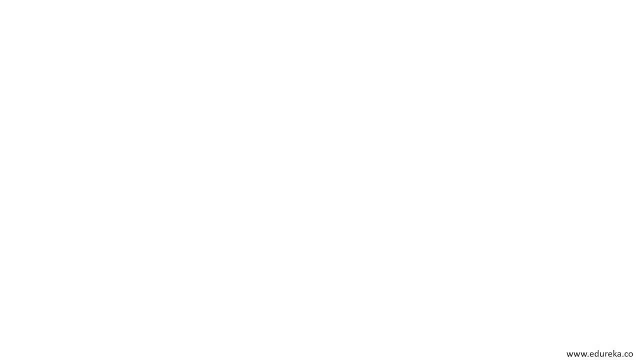 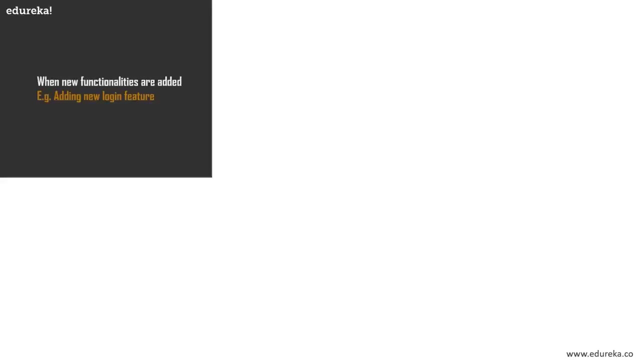 on the occurrence of following events. Let's discuss what they are. first of all, when new functionalities are added, Ideally you should perform regression testing after making any changes to the code. For example, a website has a login functionality which allows users to do login only with the email. 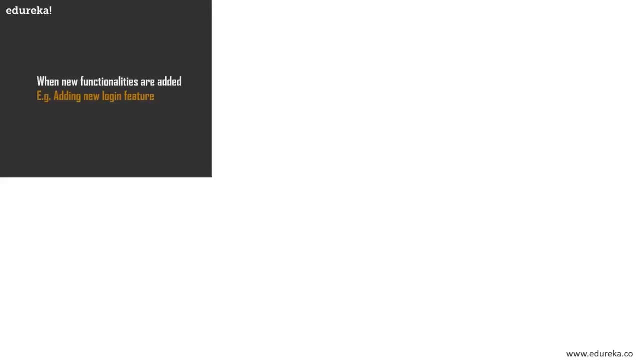 Now you add a new feature like Facebook login, So you need to check the entire login functionality of the Facebook. just like the simple e-commerce website payment option which we discussed earlier, We need to make sure that the new payment option, or, in this case, the new login feature hasn't affected the old login functionality. then you apply regression testing when there is change requirement- or usually you call it CR- in the market. For example, whenever you log in, there's this option which pops out, right? Do you want the system to remember the password? 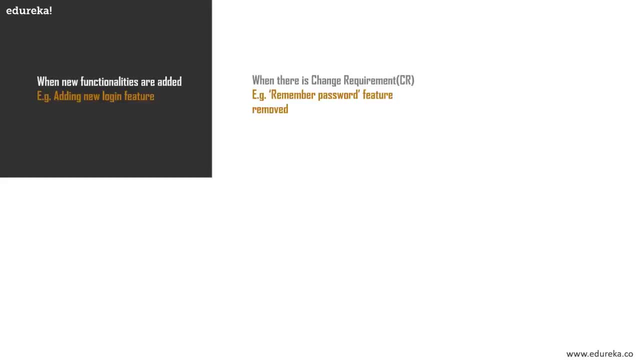 I'm sure you've seen that, so remember: password should be removed from logging page, which was available earlier. that's change requirement. It was available earlier, but you want to remove it. That's when you can apply regression testing to see if the removal of thing 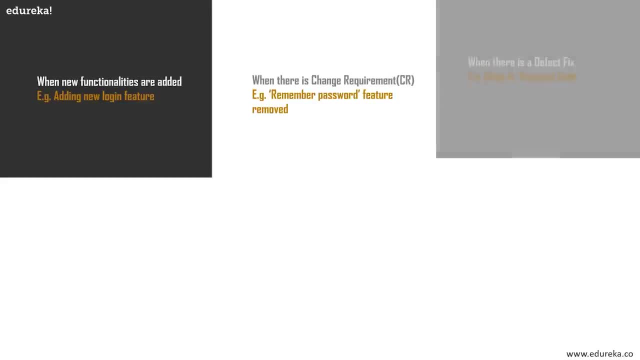 has affected the website that you're using in any way and then you can apply regression testing when there is defect. fix that straightforward. You already know that. imagine: login button is not working in login page and the tester reports a bug stating that the login button is actually broken. 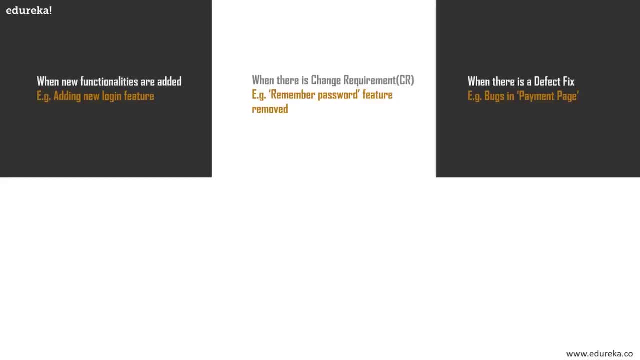 So once the bug is fixed by the developers, tester test it to make sure whether the login button is working as per expected results or not. simultaneously, tester test another functionalities which are related to login button. I like registration or any other features which are directly related to login functionality. 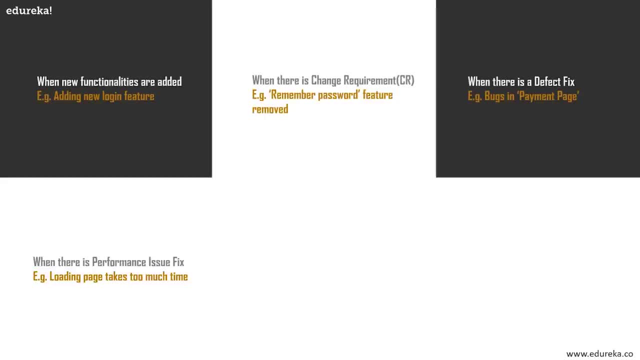 and then you can apply regression testing when there is performance issue fix, for example, when there's modification of code based on your needs and requirements. you've made some changes to the code and since then the loading home page takes 5 seconds. You want to reduce the load time to 2 seconds. 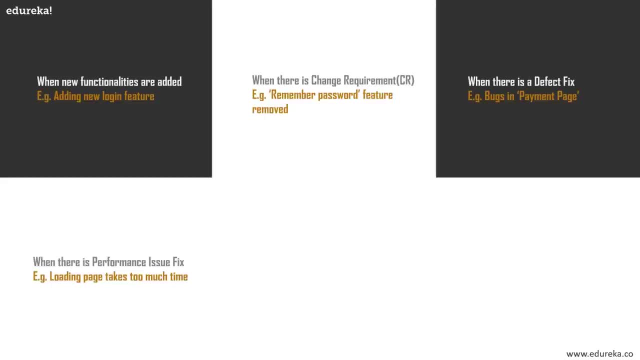 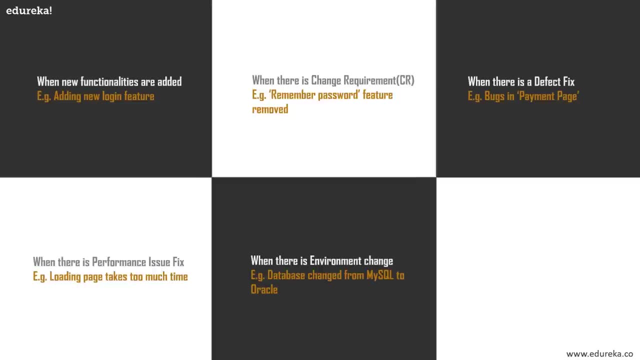 and you have done it, but you want to see if this has affected the functionality of your website in any other way. you can also apply regression testing. when there's an environment change, for example, when you've updated the database from MySQL to Oracle, all the features which are dependent on your database should be tested. 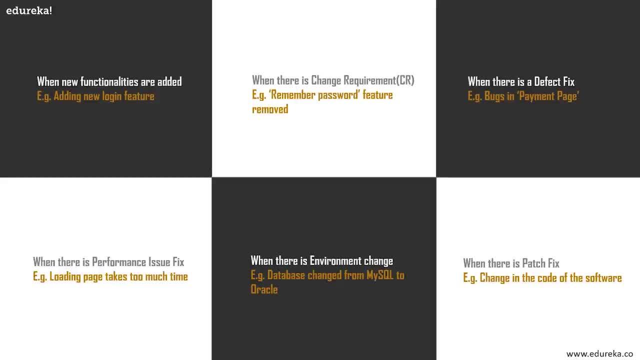 and lastly, you can apply regression testing when there's a patch fix all the mental fix problems. poorly designed patches can sometimes introduce new problems, like they can break the functionality or disable a device. So in such cases you need to perform regression testing to see if fixing a patch has actually been a profit. 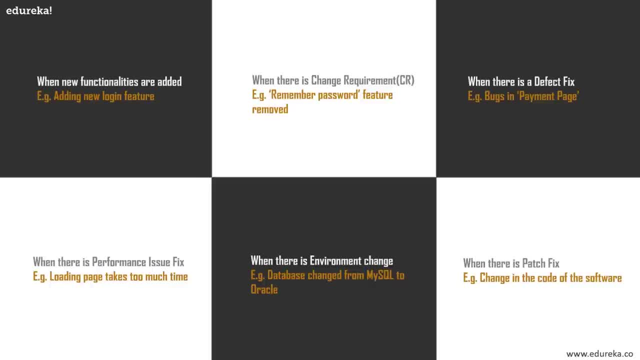 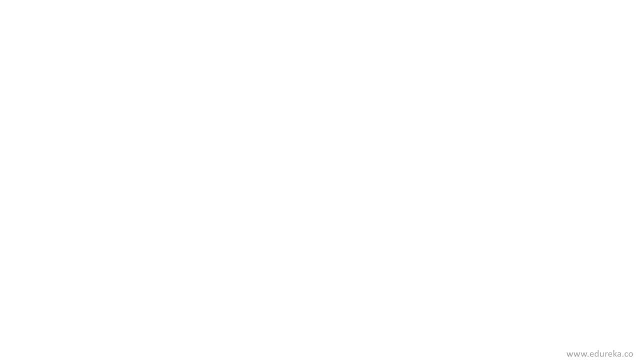 for you or loss. So, guys, these are some test cases, or you can say, situations or scenarios where you can apply regression testing and that would be beneficial for you. So, guys, often regression testing is done through several phases of testing. it is for this very reason. 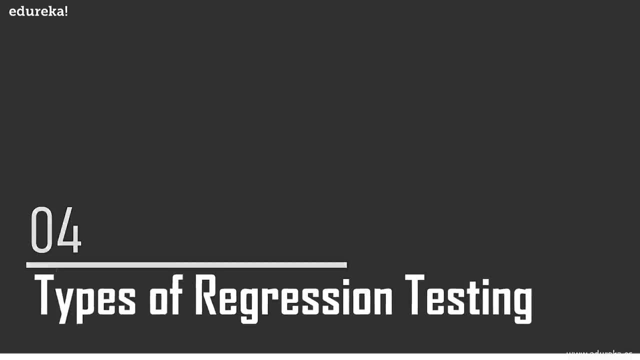 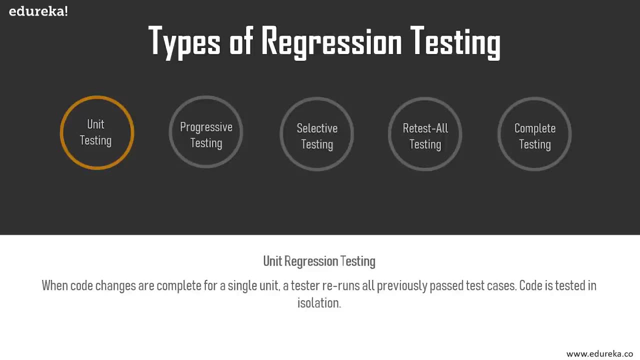 that there are several types of regression testing out there. Let's check out what they are. to begin with, we have unit testing. So immediately after coding changes are made for a single unit, a tester- usually the developer who is responsible for the code- reruns all the previously passed unit tests. 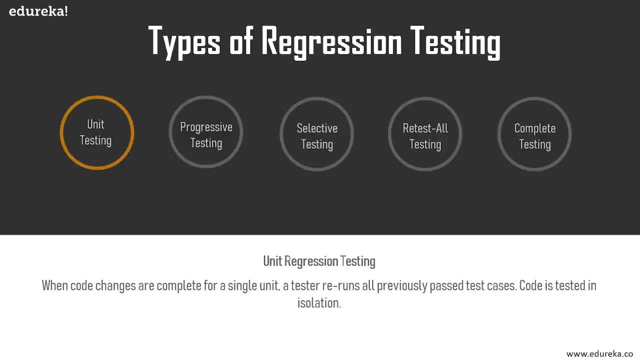 So test-driven development, which we call it TDD, and in continuous development environments, automated unit tests are built into the code, making unit regression testing very efficient when compared to other types of testing. That's what you need testing is. then you have progressive testing. 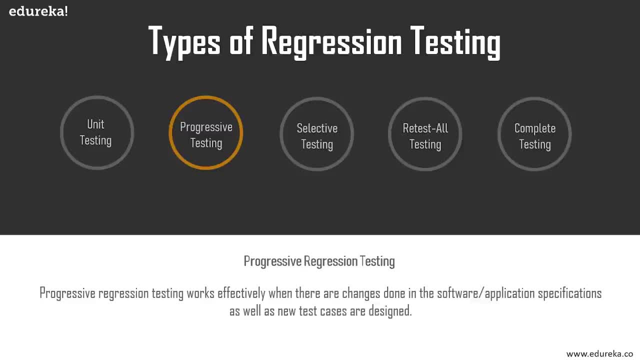 So progressive testing works efficiently when there are changes done in software or application specifications as well as new test cases are designed. that's when you use progression testing and it will be more helpful for you as well. Then there is selective testing. in selective testing, testers use a subset of current test cases to cut down the cost. 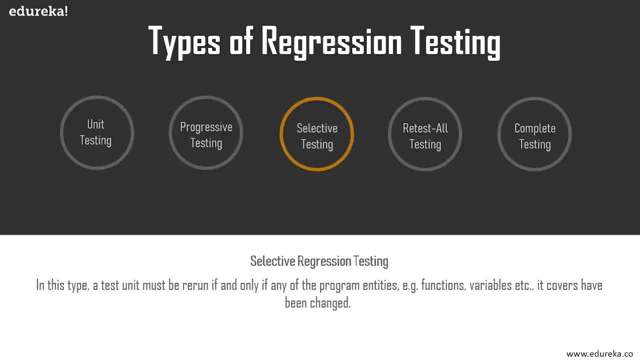 and therefore it so in this strategy. a test unit must be rerun if, and only if, the program entities, example, functionalities, variables, etc. It covers, have been changed. So basically only things like functionalities, variables which are under the unit test are changed. only then you should perform testing on that unit test. 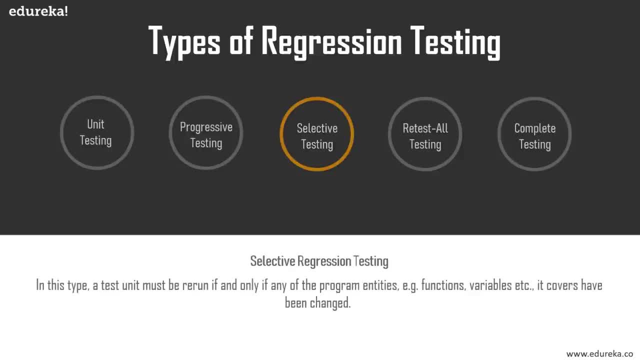 The challenge is basically to identify the dependencies between the test case and the program entities it covers. So basically, as the name indicates, you do not perform test in all units. You just select few out of those which might have affected due to change and then test those units. 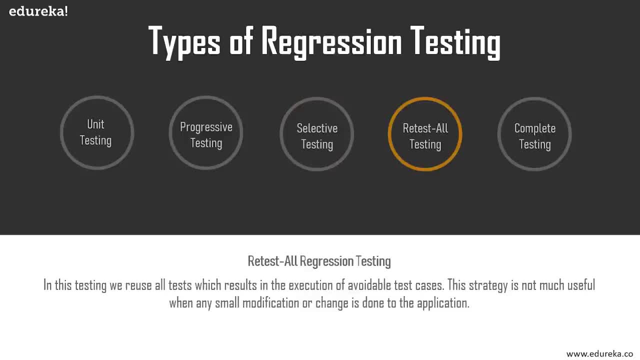 That's what you call selective testing, and then you have reset all testing. reset All testing is very time-taking because in this testing we use all the tests. This strategy is not much useful when you have small modifications or small kind of changes which are done to your code. 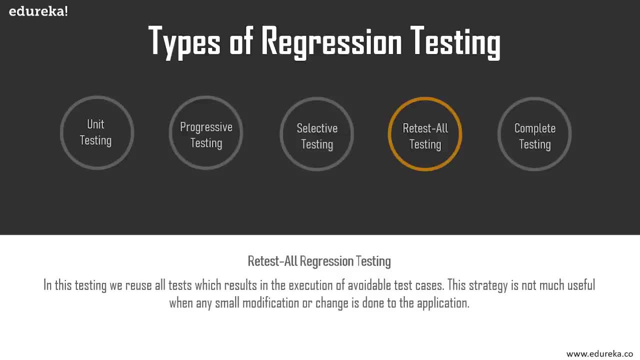 in the application you can straight away point out: right, you have made a very small change and you are trying to retest everything because of the small change. It's literally costly and it takes a lot of effort and time on your part during small modifications or changes to your code. 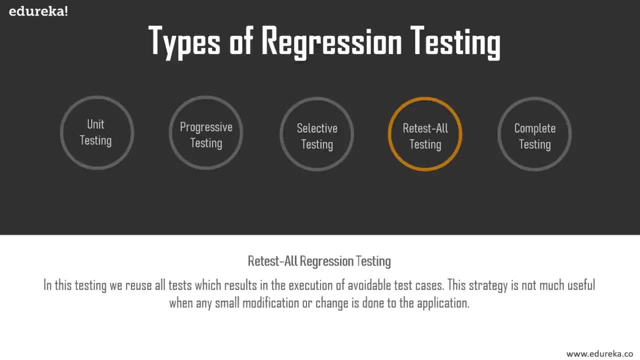 in your application, It's not effective. retest all strategy involves testing of all aspects of a particular application, as well as reusing all test cases even where the changes have not been made, So that's one of the most costliest type of testing when compared. 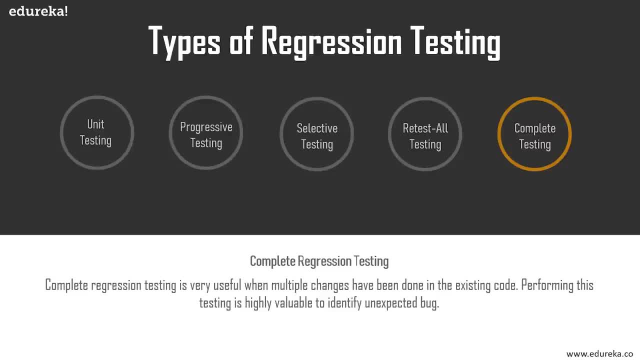 to others. lastly, we have something called complete testing. Don't confuse it with retest. all testing Sometimes people often refer to is both of them as the same thing? But anyway, complete regression testing is very useful when multiple changes have been made in the existing code. 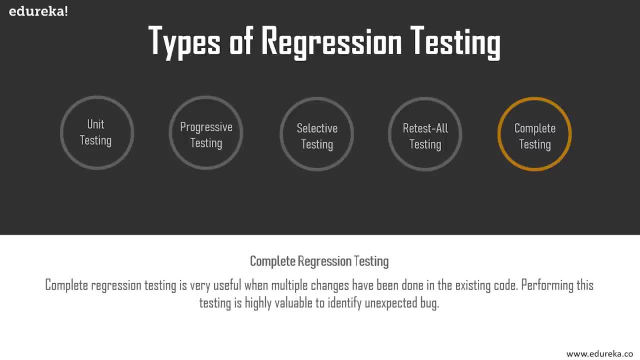 performing this testing is highly valuable to identify an expected bugs, actually. So once the testing is completed, the final system can be made available to the user. So, guys, it is important to make sure the type of regression testing that needs to be conducted, so we should choose the one. 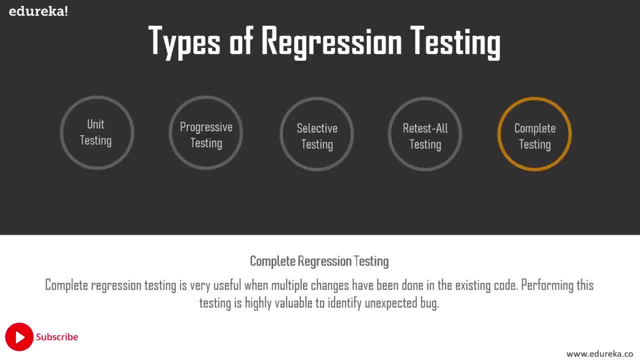 which suits your requirement properly, and how you choose, or which one you choose, totally depends on other factors such as recurrent defects, criticality of the features, Etc. But what remains on the priorities: ensuring that the software delivers the best functionality and proves to be beneficial addition. 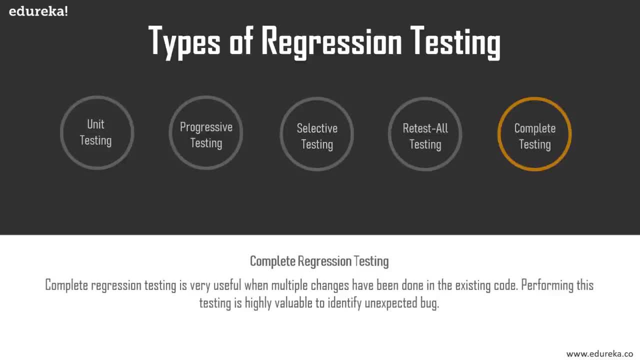 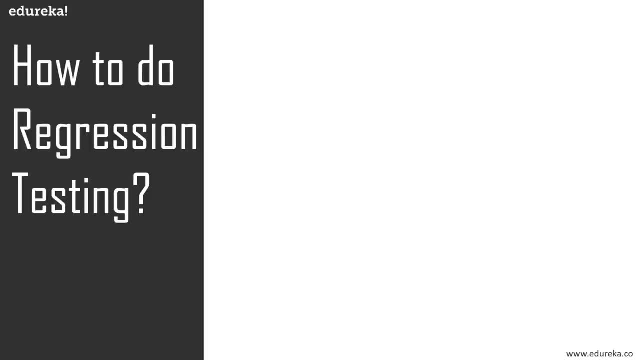 to your company or industry. So, guys, now that we have established what regression testing means, let's go ahead and check out how regression testing is actually performed. So, every time the software undergoes a change and the new version, update or release comes up, the developer carries out these steps. 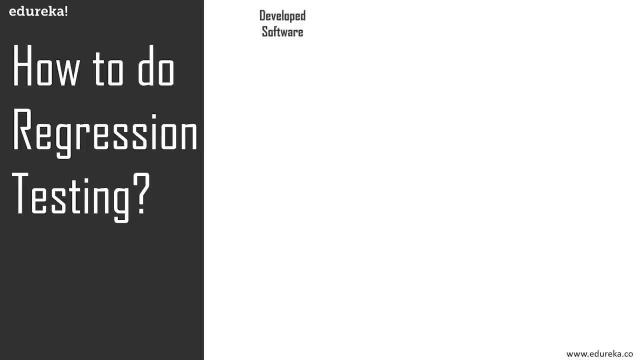 as a part of regression testing process. The first thing it does is developer execute unit level regression test to validate the code that they have modified, along with any new test that you have written to cover new or the change functionality. basically, whatever the changes that make the check. 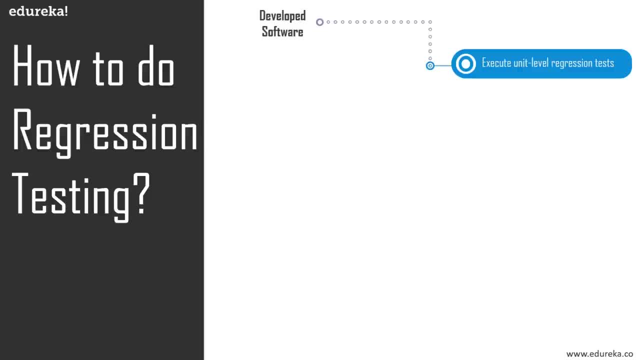 if the changes are working properly or not. So that's the first step. we did learn what unit level regression test are earlier right. So any code changes made for a single unit, a tester or basically the developer who's responsible for the code, reruns all the previously passed units as well. 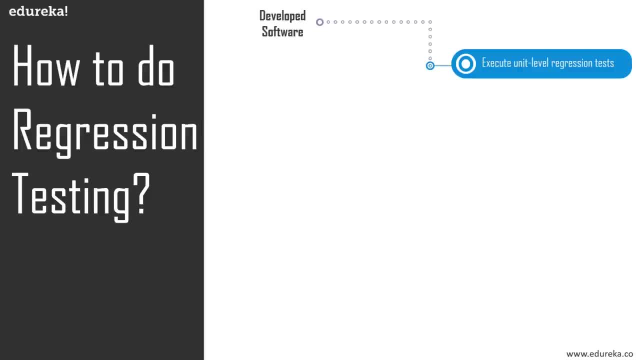 So that's what unit level regression is. once that is done, The changed code is merged and integrated to create a new build of application under test. after that smoke test upper form. these smoke tests are executed for assurance that the build which you have created in the previous step is good. 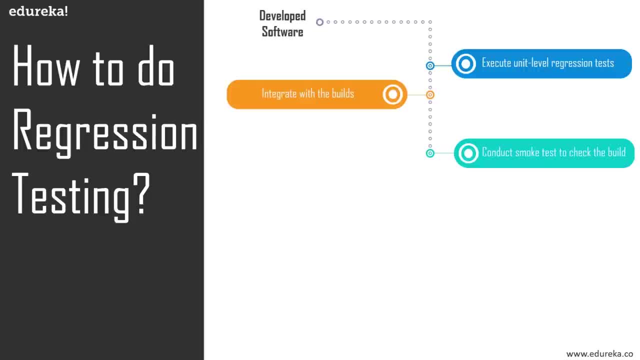 before any additional testing is performed. These tests may be automated and can be executed automatically by continuous integration services such as Jenkins, Hudson's and bamboo. So, once the build is perfect, sanity testing confirms that new functionality works as expected and known defects are resolved before any other conducting. 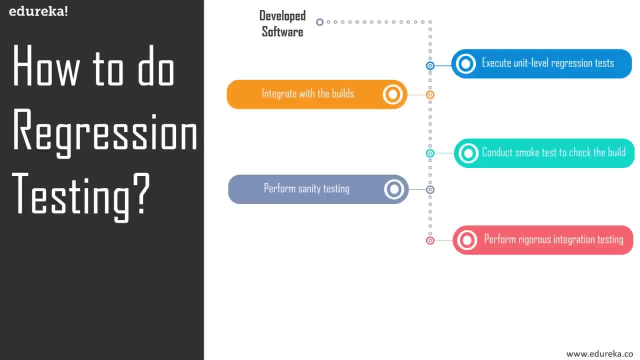 or rigorous integration testing is actually performed. So why do you perform this integration testing? to verify that the interaction between the units of application with each other and with the back-end services, such as databases, is working properly or not. for that you perform integration testing. The next step is to schedule your regression test. 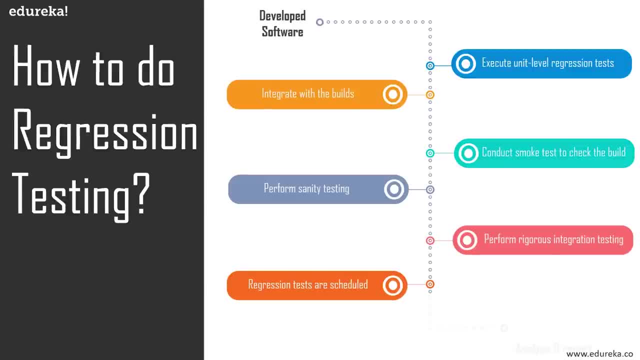 So, depending on the size and the scope of the released code, either a partial or a full regression test may take place. defects are reported back to the development team and many require additional rounds of regression testing to confirm the resolution. So, lastly, based on the reports that you've written, you analyze: 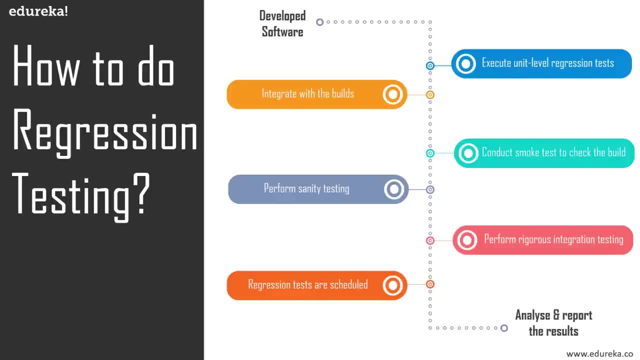 and figure out what taste cases should be added for the next checking process as well, and you create a report on that. So that's how you perform a regression testing. So, like you've seen, it's similar to any other testing. It's just that you check the functionality. 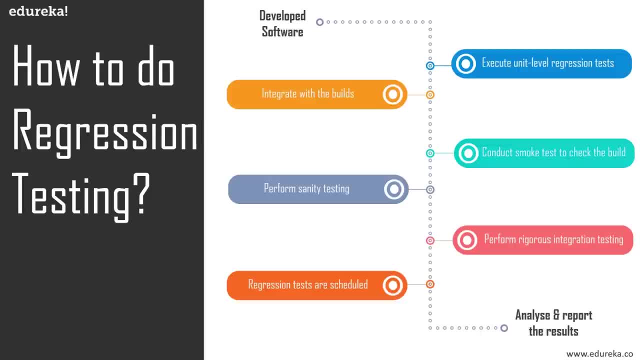 of your developed software whenever there is an update or some new release. So basically, on introduction of new feature, you check out if the previous features are working or not. So remember, guys, regression testing is not just performed in the beginning, So basically it's carried out throughout the testing process. 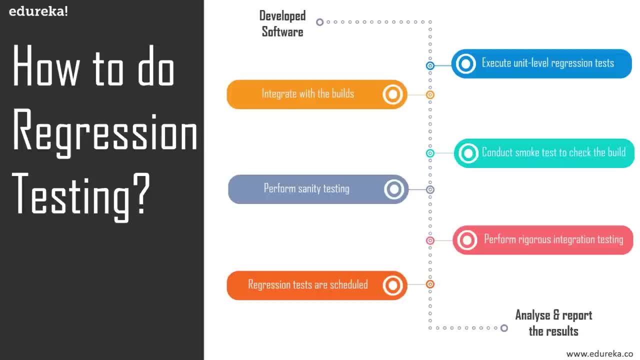 whenever a new feature is added and we discuss when to perform regression testing earlier right. So whenever one of such cases occur, we perform regression testing during the entire testing phase. So basically what you're doing here: you select the test for regression, choose a proper tool. 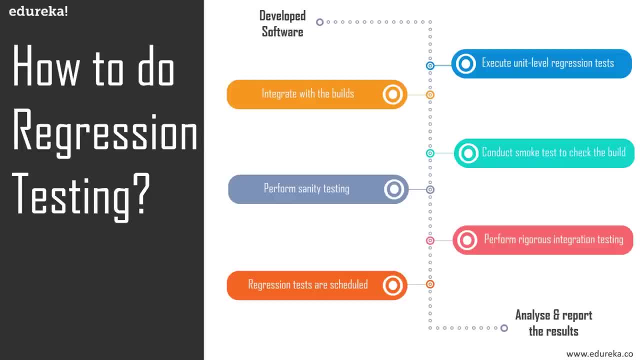 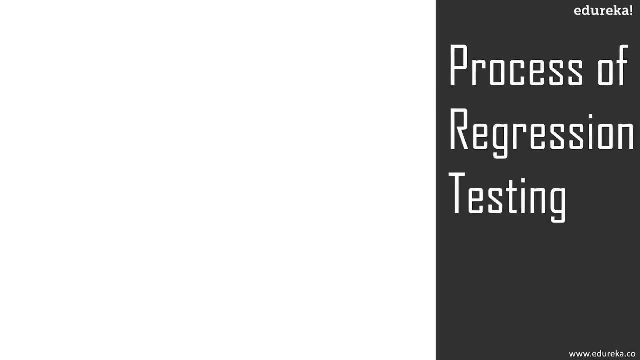 and automate the regression test, verify your application with checkpoints, manage regression test or update when required. you schedule the test, integrate the build and analyze the result. So that's as simple as that. if that was a little theoretical and if you've not understood, here is a pictorial representation. 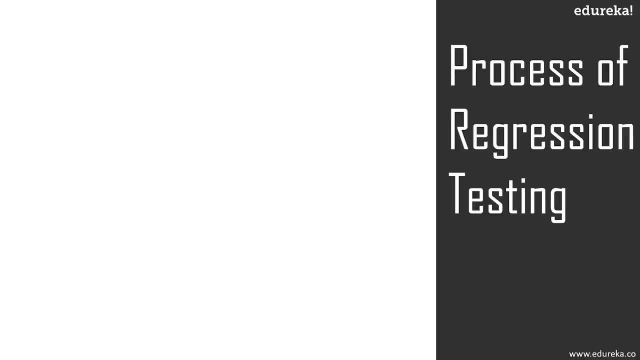 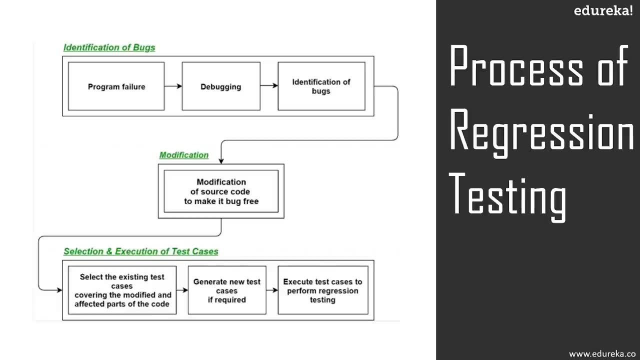 of it. So, first of all, whenever we make some changes to the code for any reasons, like adding new functionality, optimization etc. our program, when executed, fails in the previously designed test suit for obvious reasons. So after the failure, the source code is debug in order. 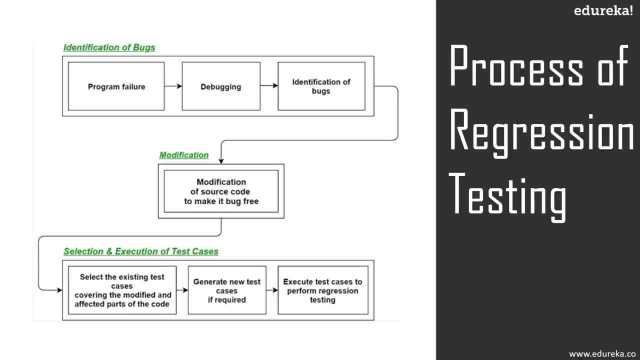 to identify the box in the program. after identification of box in the source code, appropriate modifications are made. then the appropriate test cases are selected from the already existing test suit which covers all the modified and affected parts of the source code. so we can add new test cases. 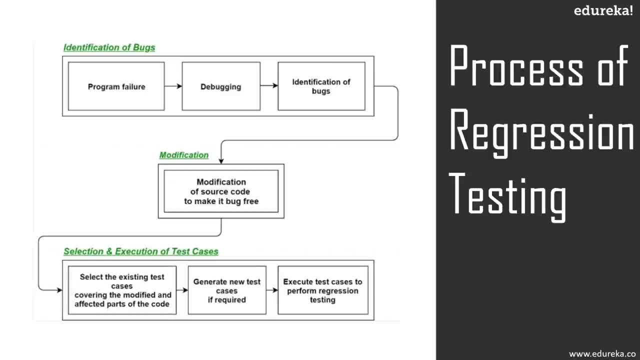 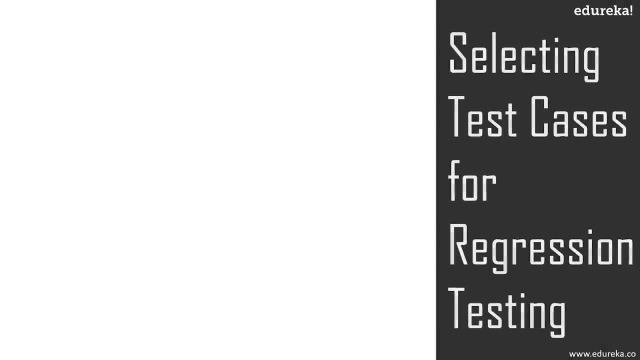 if required. in the end, regression testing is performed using the selected test cases, So selecting test cases is very important. effective regression test can be done by selecting the following test cases: test cases which have frequent effects. test cases which verify core functionality of the product. 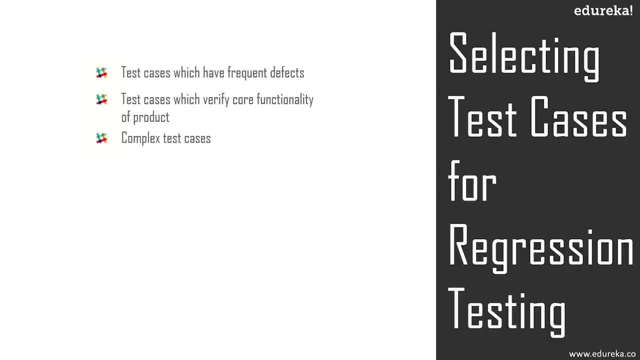 that you're checking the complex test cases, integration test cases. you have functionalities which are frequently used, So those are the first ones that you should check out. then you have test cases which cover the module where the changes have been made. Those are obvious. then test cases. 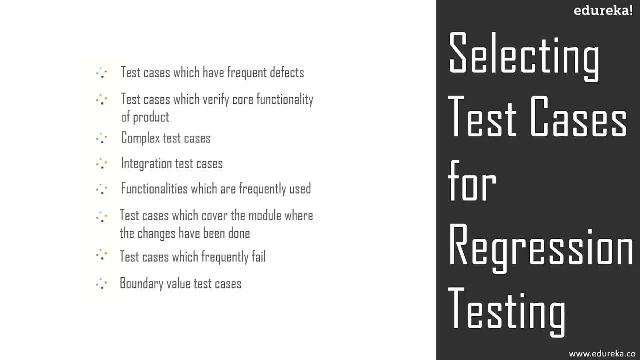 which frequently fail for no reason. then you have boundary value test cases. So these are certain test cases where you can apply regression testing, or you can actually select these test cases for regression testing. So when you're trying to shortlist the test cases for regression testing, 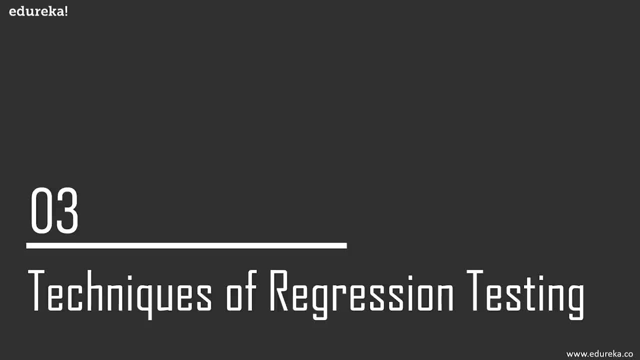 these are some points that you should consider. So regression testing simply confirms that modified software hasn't unintentionally changed, And it's typically performed using any combination of following techniques. So, basically, what I'm trying to say here is that there are three techniques that you can apply for regression testing. 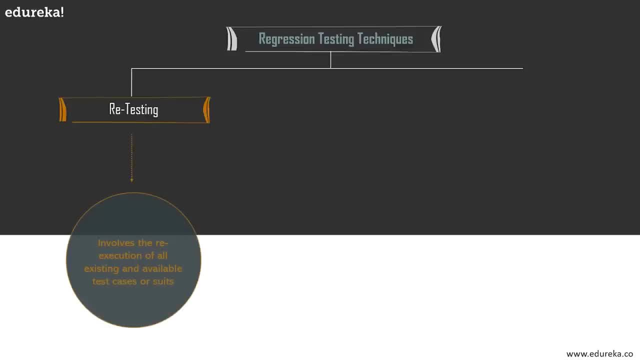 So the first type we have is retest all this method of regression testing. simply retest the entire software, so from top to bottom. in many cases, the majority of these tests are performed by automated tools and certain times automation is not necessary at all. Moreover, purely using automation ignores the benefits. 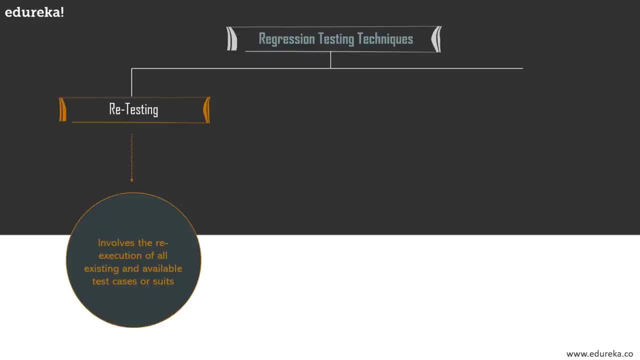 of human testers and any change for exploratory testing. So this retest, all type of technique, is an expensive method as it requires more time and resources when compared to other techniques. Well, it's all there in the name itself, right? retesting. The next is selective test cases- again from the name itself. 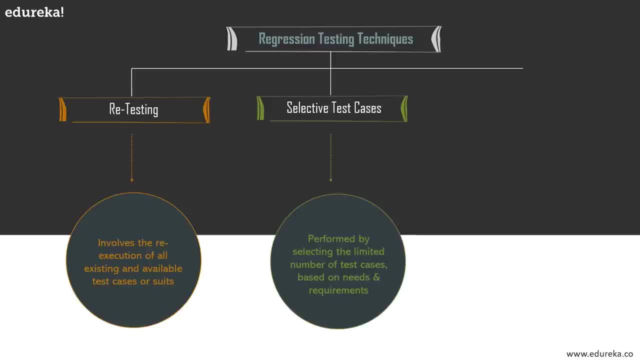 You can guess what that is. rather than a full retest process, This method allows the team to choose a representative selection of tests that will approximate a full testing of a suit. The primary advantages to this practice is that it requires far less time and effort. 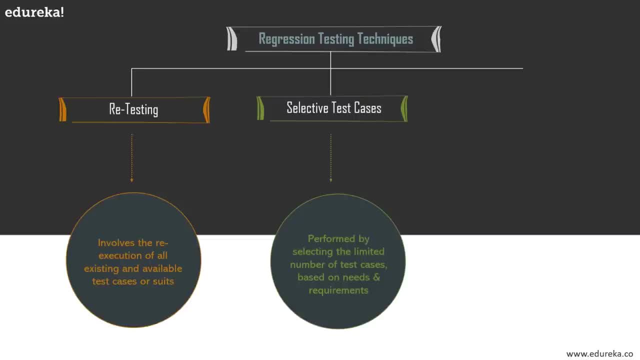 when compared to retest all method. So these kind of regression testing is usually performed by human testers, such as quality analyst team or development teams, who will typically have better insights into the working of test cases and their unexpected behaviors. And lastly, we have test case prioritization. 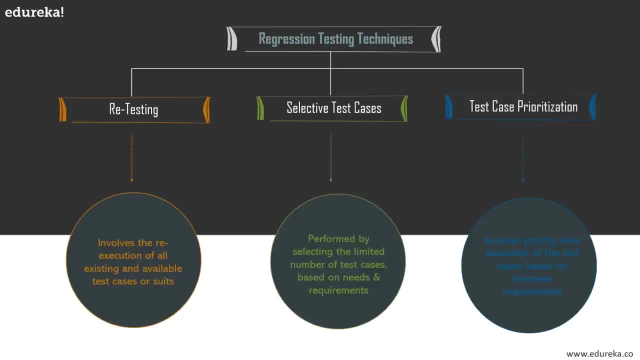 This is one of the popular technique. The goal here is to prioritize a limited set of test cases such that more potentially impactful tests are executed ahead of all less critical ones. So try to prioritize test cases which should impact both current and future bills of your software. that way you're not wasting your time, money. 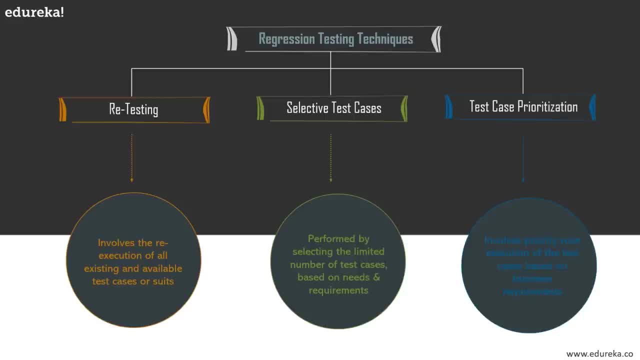 and effort. apart from these three, We have another one called hybrid. hybrid technique is literally a combination of regression, test selection and test case prioritization. So, rather than selecting the entire test suit, select only test cases which are executed or re-executed depending on their priority. 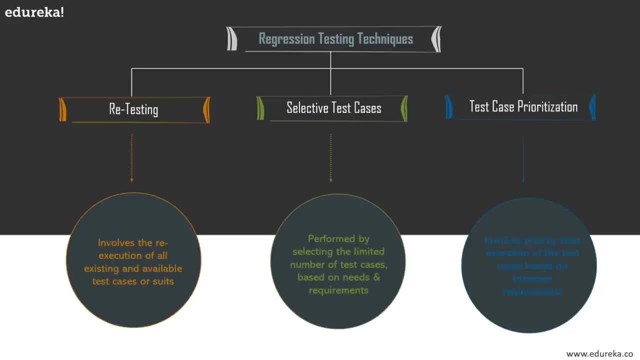 So what are the different techniques We have? retesting, where you perform testing on the entire test cases that there are. then you have selective test cases based on certain criteria. You select the few test cases. then you have prioritization: you select the more impactful test cases compared. 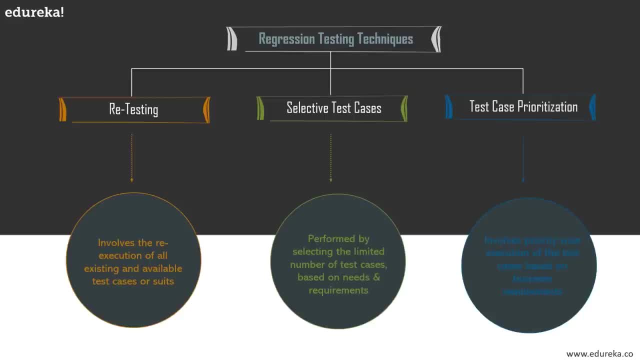 to less critical ones. and lastly, the hybrid, which is combination of selective and prioritization. So these are various ways of implementing regression testing. guys, Now that we know what regression testing is, its types and its techniques, Let's go ahead and do a demo on how to create. 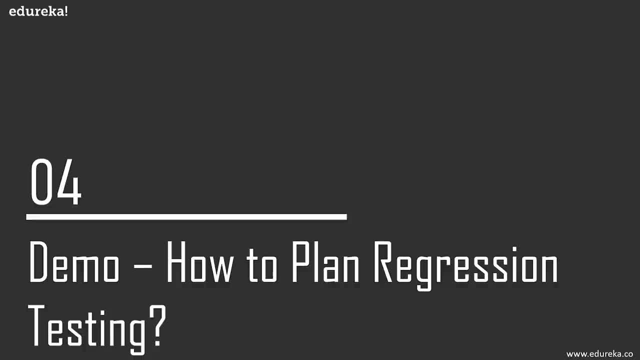 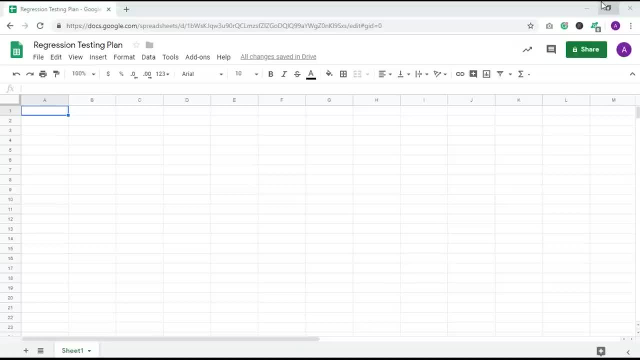 a regression testing plan. for that I'll be using an excel sheet. So, guys, here we are. in this demo, Our main goal is to actually learn how to create a regression testing plan. It's a very simple example. So, with this example, 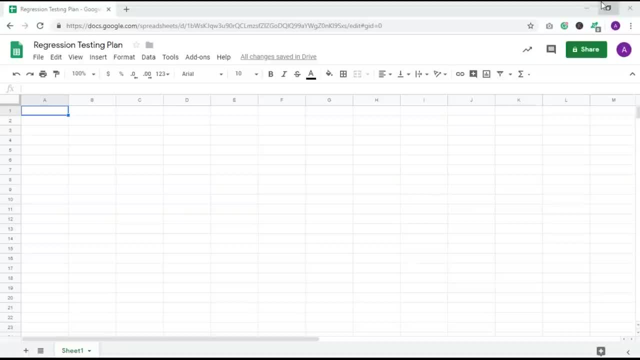 I'm sure you'll be able to get started on how to perform regression testing. So, first thing, there are certain terms that you should know about. as for this regression testing plan will be using an e-commerce website to test on or to create a plan actually. 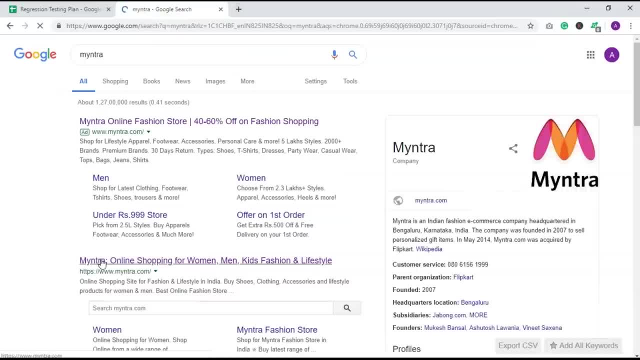 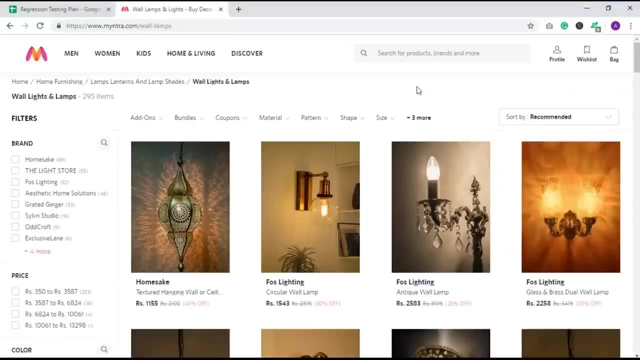 So let's take mantra: Here we go. Okay, what do I want to see? So we go. I'm choosing wall lamps and lights, anything just and basic example to check on. let's perform or create a regression testing plan for the sort option here. 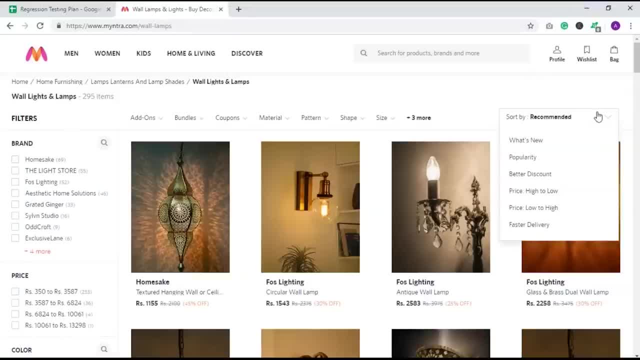 You can see right the start here. when you click on that You have different options like sort, the elements based on what's new popularity, better discount price, high to low, price low to high and faster delivery. So we'll be creating a regression testing plan on that. 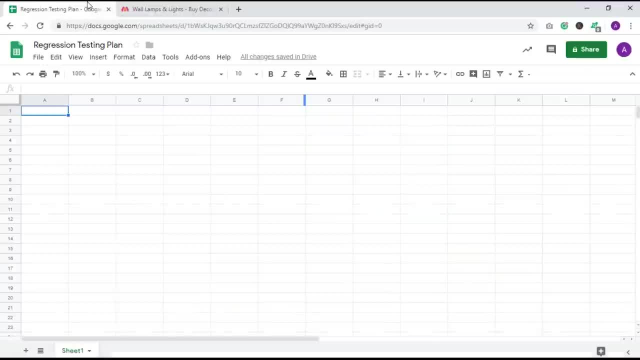 Let's go back to Excel sheet. Like I said earlier, there are certain words or terms that you should be aware of. the first thing, Let me just write the headings first, Let me increase the size, then we have what they mean, and then comes our example. 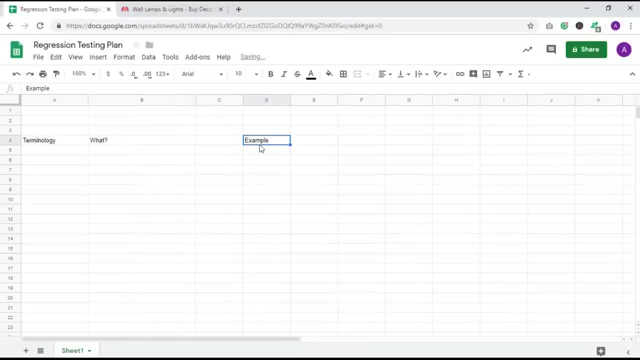 Okay, let me increase the size of this one as well. Okay, first terminology is test objective. So what does a test objective mean? It's basically what you're trying to do here in this. We're trying to test a functionality of your feature. 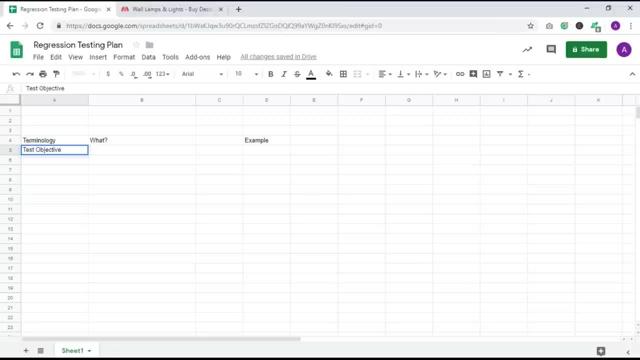 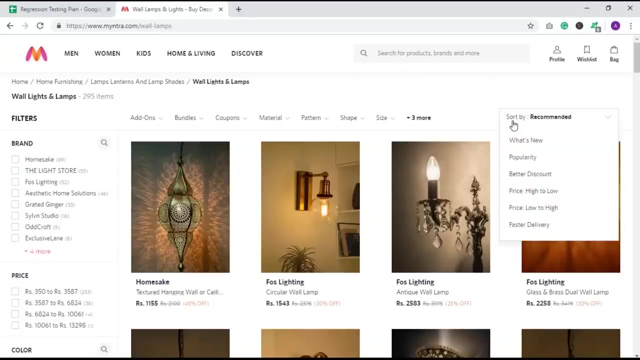 That's what your objective, the goal or the objective of creating this plan. That's what we call test objective, So you can say what you are planning to do. So what would be the example here with trying to check the functionality of a feature, here trying 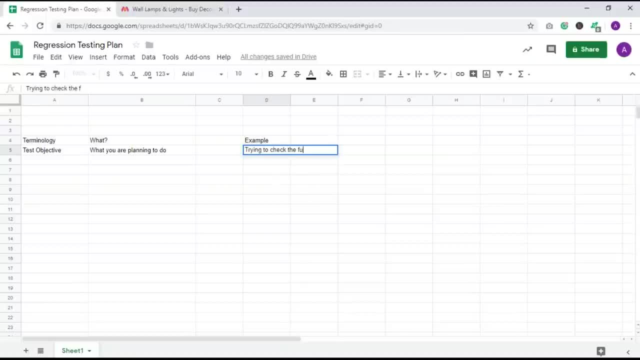 to check a check the functionality. The next term is test object. So what do you mean by test object? It's basically the component which you're perfect test on, but performing test on, so component to be tested. So what's the component that we're trying to test here? 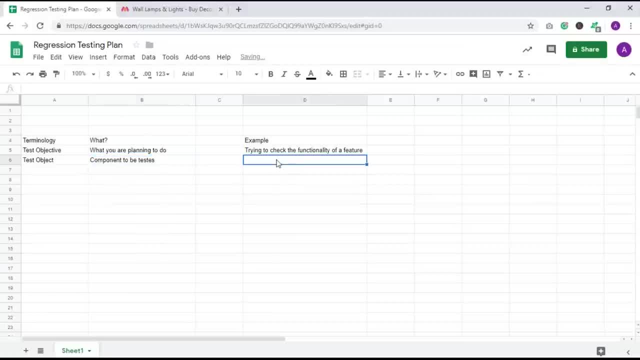 The sort components. So that's our test object. So I'm going to say sort feature. So we are done with test object and test objective. We have something called test item next. So what's in test item? This item is the subset of your test object. 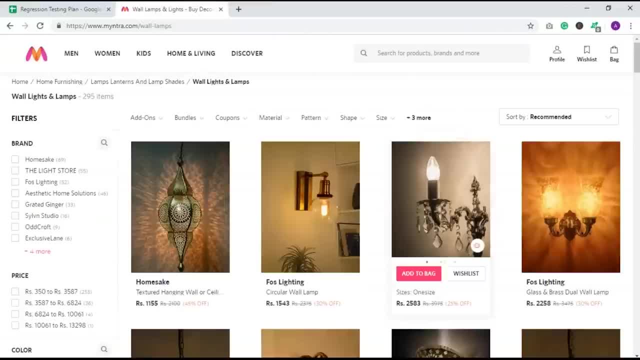 or the item that you're performing test on. So this is the object that we are performing test on, which is sort. like I said, under sort We have multiple options. So these are nothing but test items here. So let's say, let's perform a test on this price high to low. 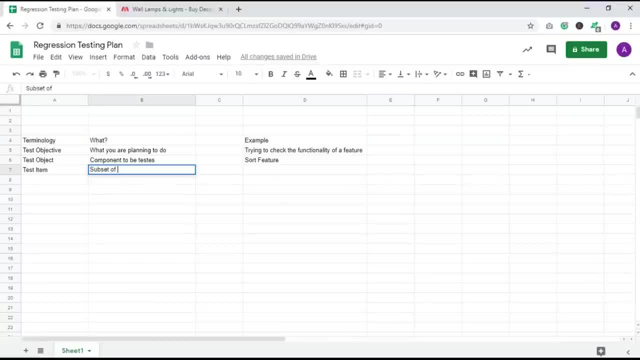 So let me write it as sub set of test object. So what are the item that we are checking here on price, From high to low. The next thing is test condition. So under test items, like I said, it's a subset right. 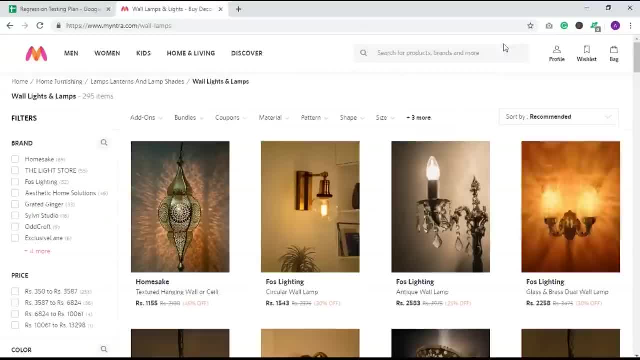 You can have any number of items or subsects for an object. For example, like we said here, we have what's new popularity. and also, let's say, if I want to select two options or two objects or items that I want to check here, 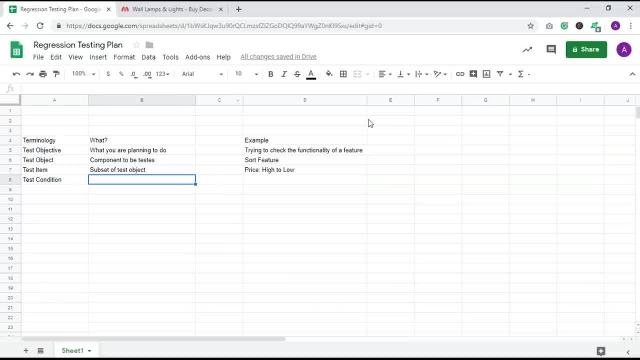 which is price high to low and price low to high. I can add both of them here: high to low, comma, low to high. So the test condition is the one thing which you're testing of these items. So let's say we want to check the sorting feature. 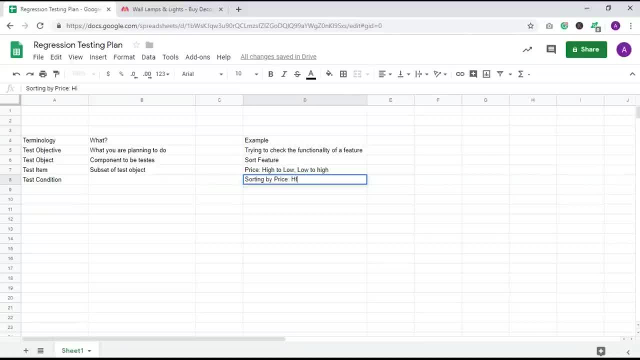 by price, high to low. So you get the point right, basically the condition on which to performing testing, and then you have test case. test case are just parameters that you can relate to when you're actually performing testings. For example, you have test data that you're checking on. 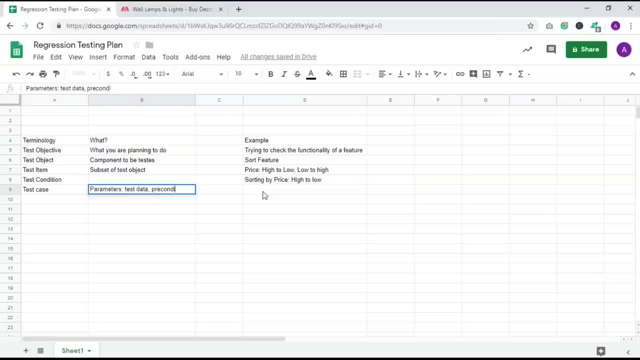 then you have preconditions. If you do have any, or you can say assumptions, and then you have expected results, Actual results of testing and all that. So, guys, if you want to know more about his cases, there's separate video by edureka on test case. 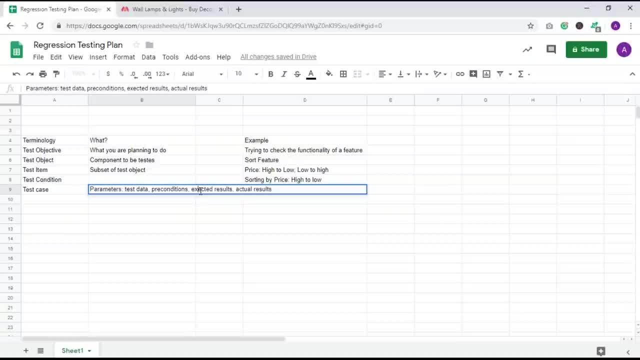 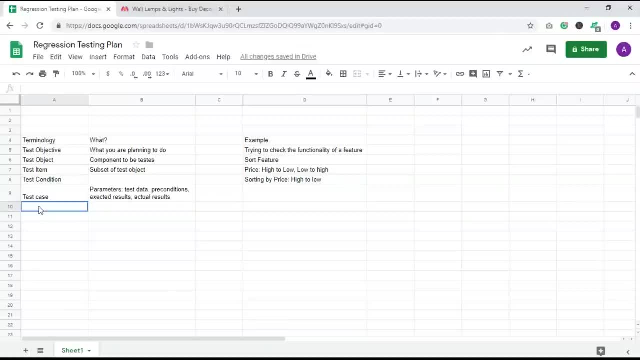 It's in the software testing YouTube playlist. Go ahead and refer to that. So yeah, I don't have to give you an example, right? So I'm just leaving it blank. And lastly, you have test suit. This with is nothing but a combination. 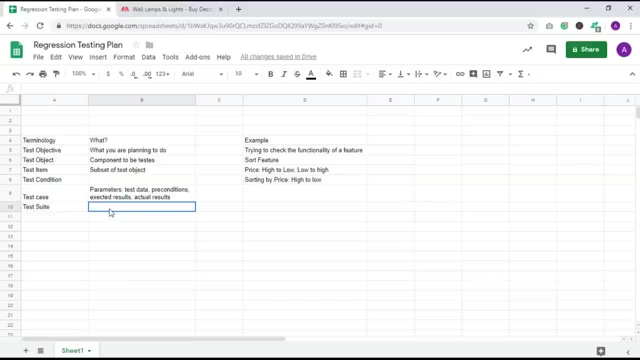 or collection of test results that come under test suit so I can write it as set of test cases. So these are certain terms which you should be aware of when performing a testing or writing a test case, or when you're creating a regression testing plan or anything. 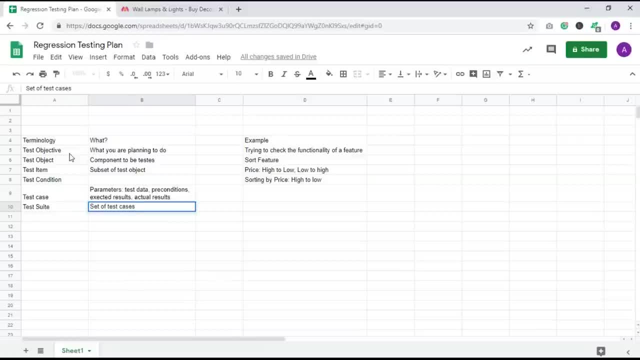 So the first thing is test objective: is your goal or think what you want to do? For example, here we are trying to check the functionality of a feature. Then you have something called object or the feature on which you performing test, on sort feature, on the soft object. 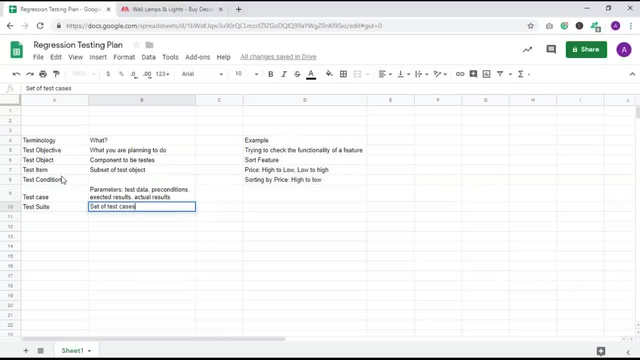 You have multiple options. those come under your test item and the test condition is based on what condition you're trying to check your test object under which a test item comes. So basically, we're trying to test out the sort feature based on price and high to low. 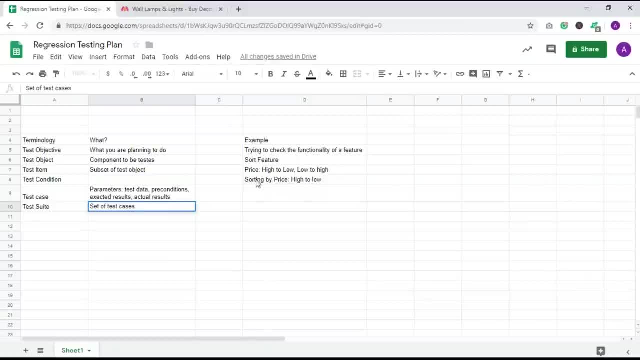 So in test condition you have three things. you have your test objects, which is sorting by the item, which is price, and an item which is high to low, and then you have test cases. These are like certain parameters which are associated when you're performing it like test, like test data preconditions. 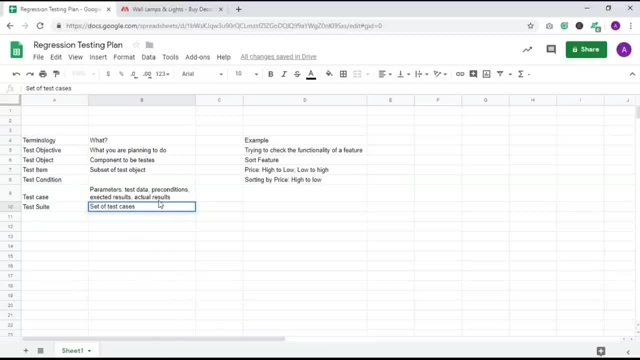 If you have any expected results, actual results or any other comments, status and all that comes on your test cases. And lastly, you have something called set of test suit, which is set of test cases which come under the same category. you can say: So what are we trying to test? your testing project name. 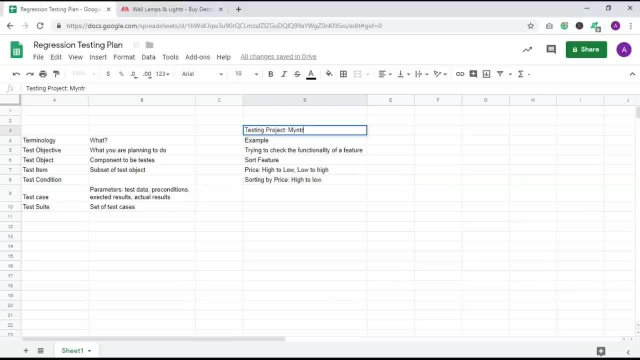 Let's give it a name which is mantra release one. Let's say so for this first release one: Let's write something called traceability Matrix. This traceability Matrix basically helps you keep track of how you performing testing on and what, and what are the results. 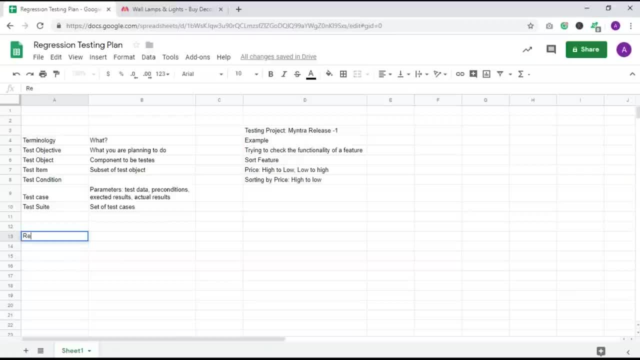 So here we have traceably Matrix, Let's say for release one leac, release one Traceability Matrix. the first one is feature, or you can just call it test item. Then you have requirement ID, Then the test suite, and then comes the test cases. 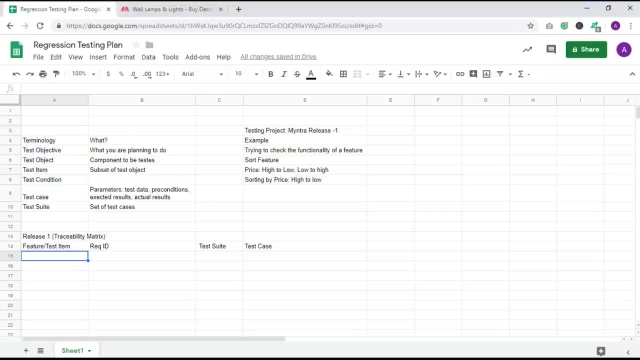 So we go, let's try it. the first element here, So that would be: this is the website that we're testing for, and what are we testing? the sort feature That's the object and the item is price, price. And what is that We're testing for? let's take high to low first. 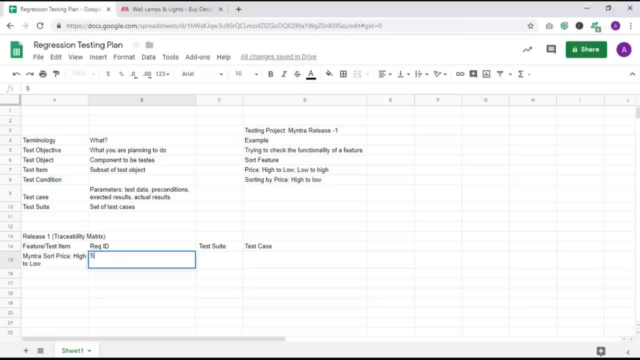 Then requirement ID, some number you can give. so we're testing sort feature. So let me give SF and 077 test suit 20.. Then the test case ID. That would be a mantra sort price which comes under the requirement SF 077 and the test case ID would be test C 0, 1.. 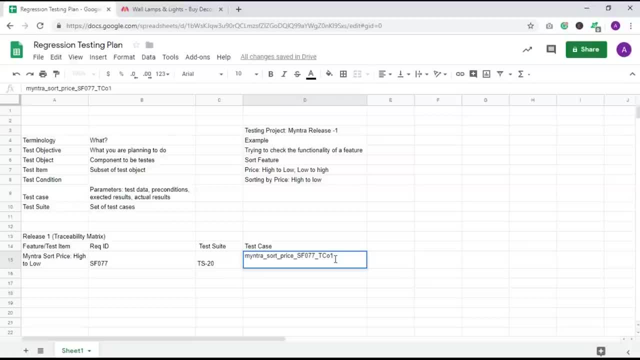 Let me give the this cap, this test case 0, 1.. So yeah, just like that, I can create multiple test cases: 2, 3.. So here we go, We're done with the first traceability Matrix, the first element. Similarly, you can write: 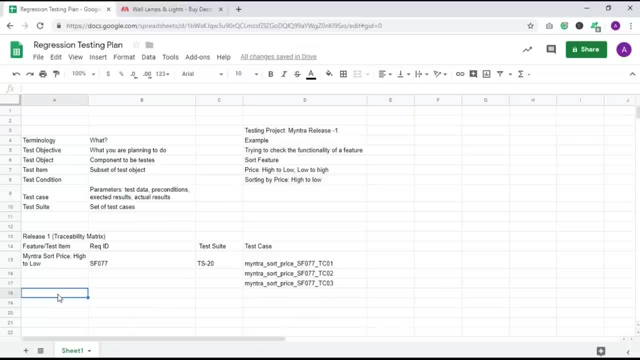 one more for low to high as well. I'm not going to write it, It's the same. So this is how we write a traceability Matrix for the release one. So let's say, you have performed testing by considering the filter option, which is high to low. 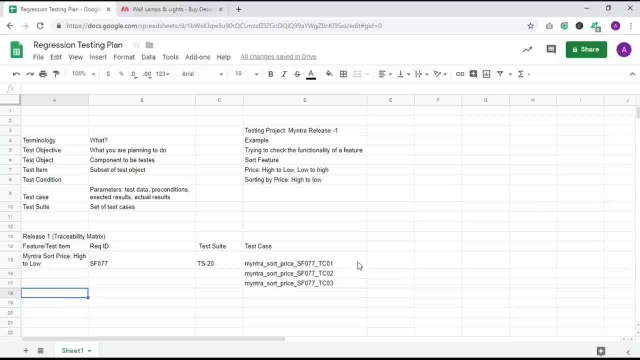 and the testing work properly without any errors. and these are the test cases which you have checked for high to low, and everything is working properly and for now it's good. novel. move on and perform testing for other feature, Let's say another item actually with it, perform. 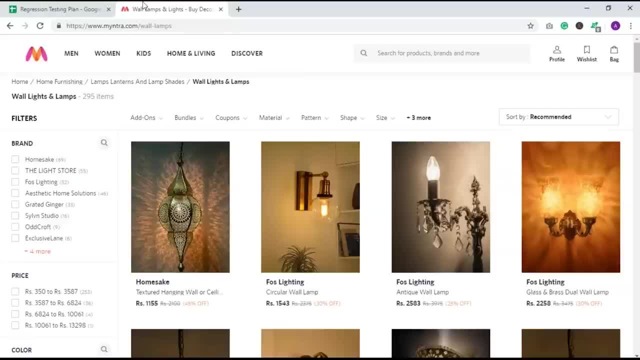 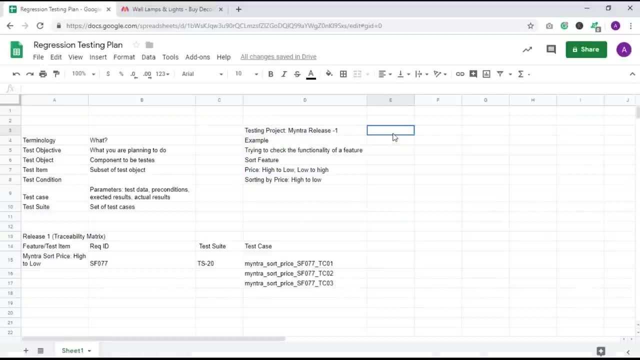 for high to low. Now let's go for better discount. You can see the better discount option here, right? So I'm going to perform test for that. All right, it is planned for that, So it's the same thing again. 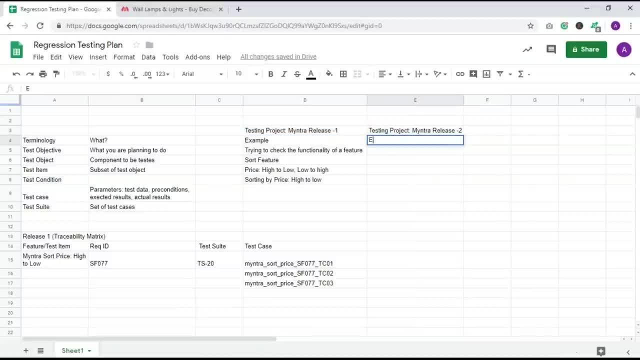 So testing release. This is example as well. It's the same. So I'm trying to still check the functionality of the feature. So my objective is same. and what is a feature that I'm trying to check on? sort feature I'd again, it's the same. 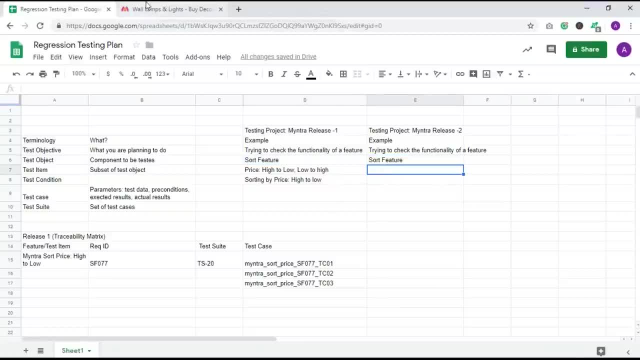 and what is the thing I'm trying to check on? It's not perfect. Surprise. now it's discount, better discount, and you do not have any multiple options here, So it's just better discount. So there we go again. We have test cases, multiple test cases. 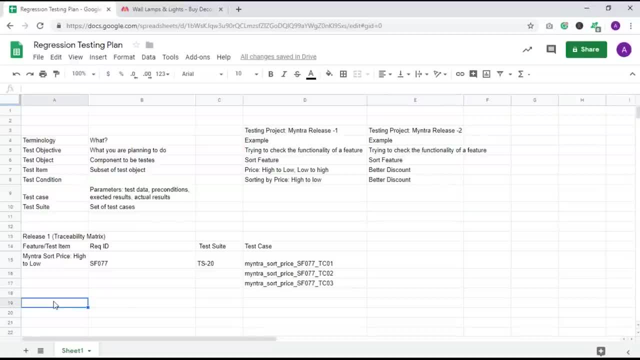 and that and multiple test use under that. So let's write a traceability matrix for that as well. SF 076 and test suit 32. that will be sort discount and the test requirement ID, which is SF 076 in this case, and then comes the test case ID 01, just like that. 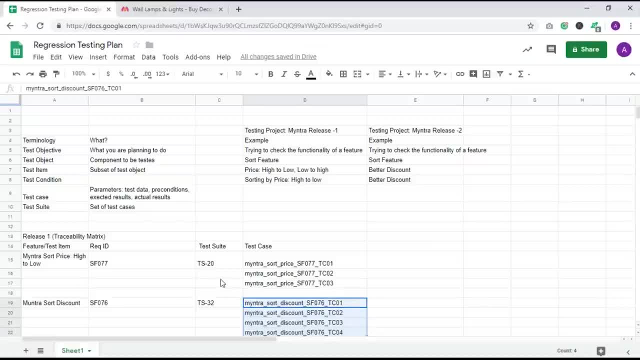 But here I have four test cases. So that's how you write your traceability matrix. Then now you're still dealing with the normal testing process. Let's move on to regression testing. Now what happens is, when I tried to test on this feature, 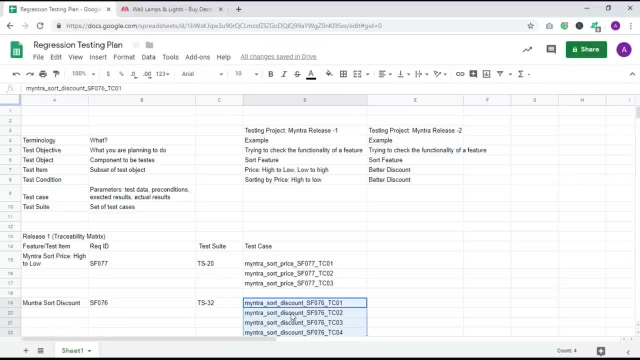 it's working properly. Then when I tried discount option, it's working properly. But after I added this discount option, when I try to check for price again, I want the sorting being done from high to low, but based on discounts. then this option, which is high to low, is not working properly. 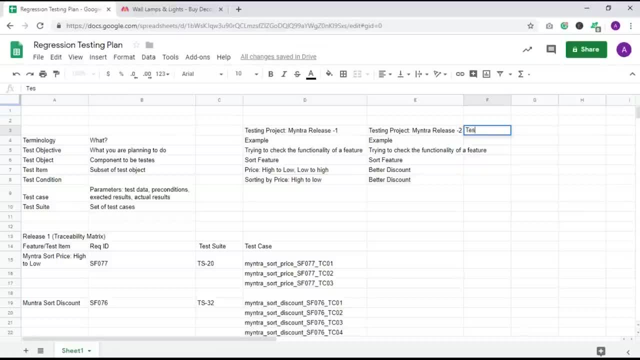 So again, here I have a testing release which is still do. I'm just going to drag it from here. Let me increase the size of this I'm still into. it's just that after introducing the new feature or the new functionality, the previous functionality stopped working. 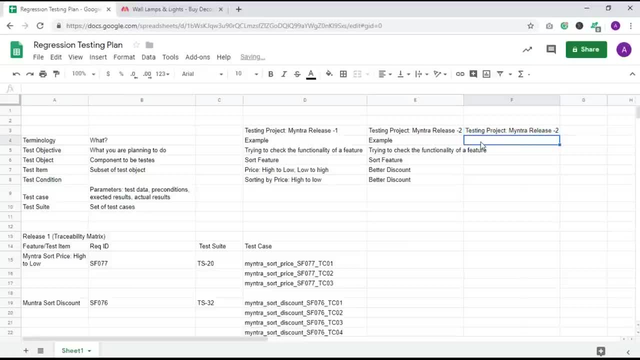 or have gone away. What an error. So it's still example. For what is regression testing? What are we trying to do here? trying to check the functionality. but we're performing regression testing, So that's our objective. So what's the feature that sort again. 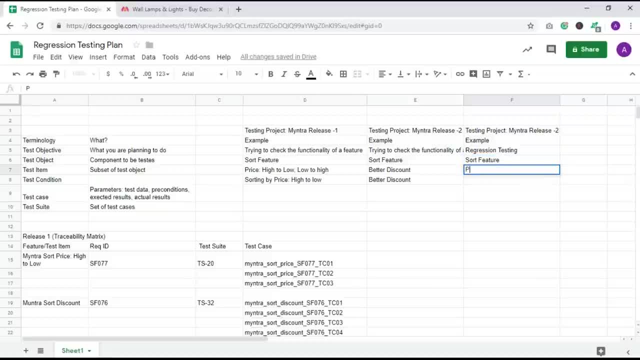 We're still checking out the sort feature. What is the thing that's not working price? High to low and low to high. So I'm sure you're understanding right. This is my only feature which was there in the sort consider. I tested it. 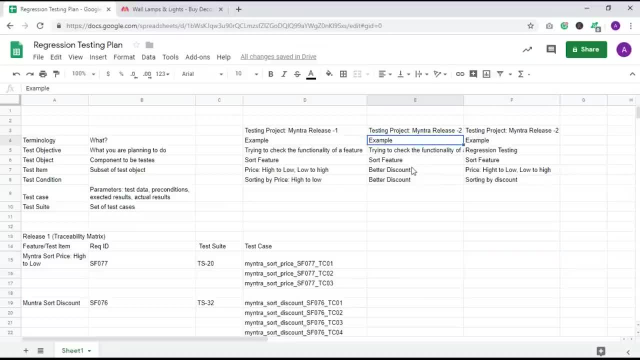 It's working properly. This also is working properly. the second one, which is based on discount. but I'm trying to win. combine this and see how the high to low is working based on the discount. The high to low thing is not working. That's when I want to perform regression testing. 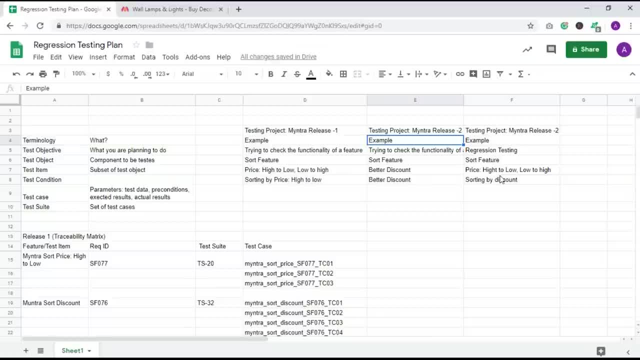 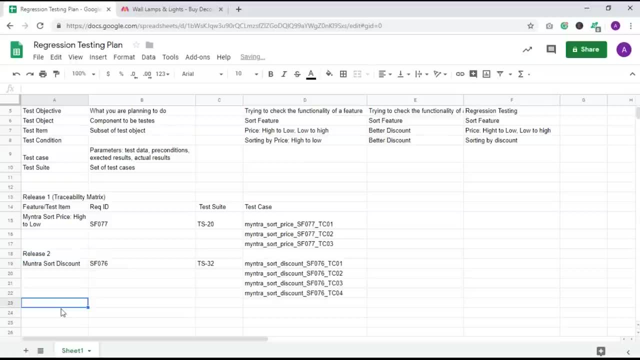 and check out what the test cases which are not working and what are the bucks. So that's how I perform. for that I'll be writing under the traceability Matrix. This would be for the release to. this is again for the release to itself. 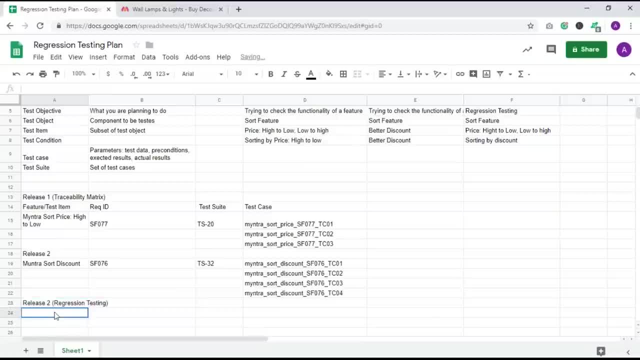 but for the regression testing, Here we go. The first thing that happened was that the defect that we found. So the first option would be, or the parameter would be, defect ID, And let's say the defect was some number 245 E. So what was the test case on which the if a defect occurred? 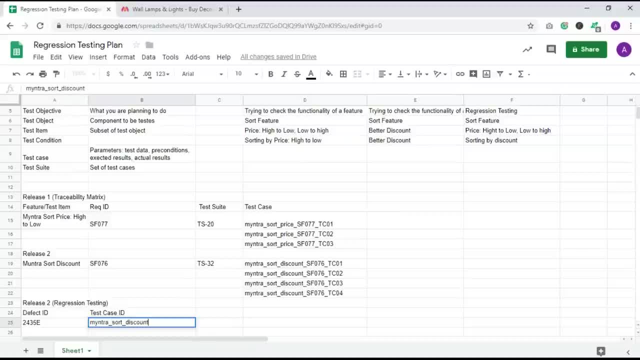 That was Myntra sort discount. So, performing the test suit, give it a number, Let's say it is suit 34.. So the requirement ID next: Myntra sort. when we try to combine the price and this can't, we got that error. 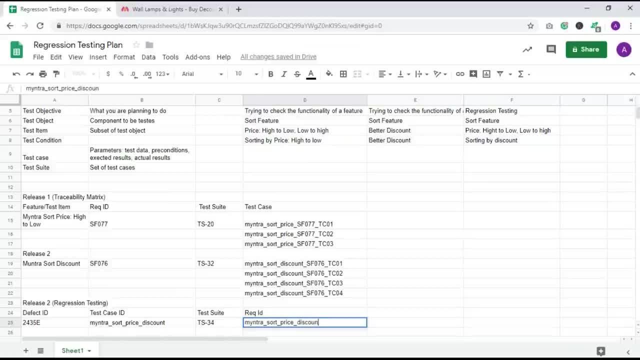 So that's it, Myntra sort, price discount and the requirement ID, something we should give right, Let's say SF 0 or 98.. So then comes the test item or the feature. Now you might be a little confused because the format which have used in the first 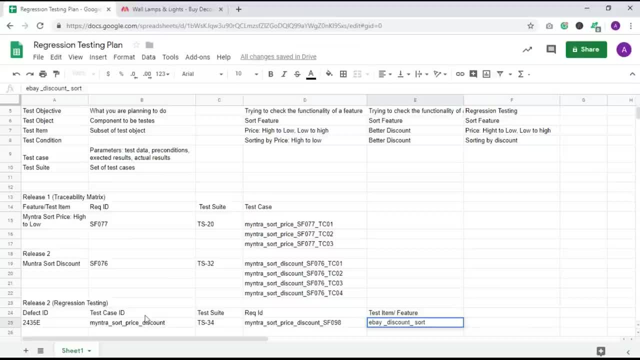 and the one which have used now is totally different and it seems a little weird. Let me go through it again. So here you have something called a regression test cases and regression test suits. So basically, guys, these matrix, We call it a bi-directional traceability matrix. 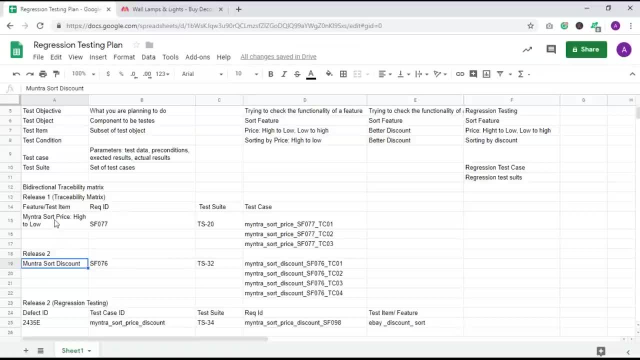 So the first one. let me just go through it again. The first one: we have your item on which we're sorting the requirement ID, the test suit which the test case belong to, and these are the test cases which come on the test. So now, what we did is we perform testing. 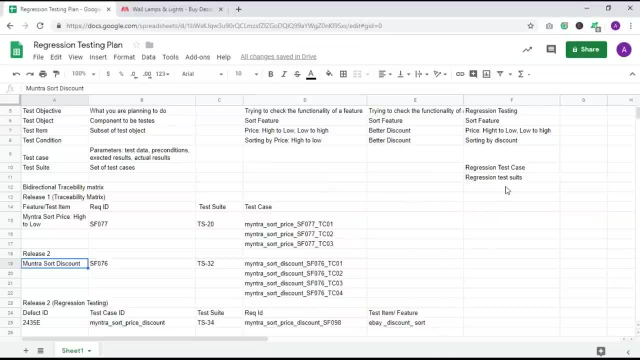 for both the features and when we try to check if combining this features or the functionality of high to low is working after the discount feature is added, It's not working. We are getting an error or a defect and that effect, as a Heidi, that defect ID we representing here. 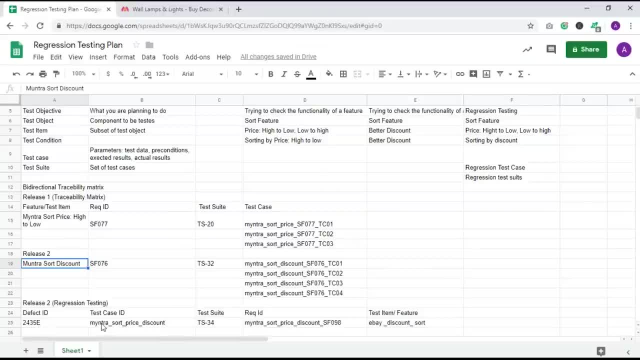 So, but when did we get that here? So what is the test case that we did test for here? when we try to sort first based on the price and then apply, the discount thing is not working. So that's the test case ID. And which test case does this test case ID belong? 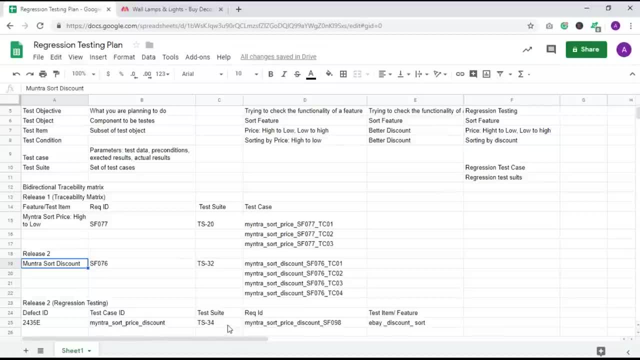 to this particular test suit and what is the requirement of this particular test case, sought based on price and then on discount, and this is the requirement ID. So what is the item or the, basically the feature or the object that we're checking here on sort? 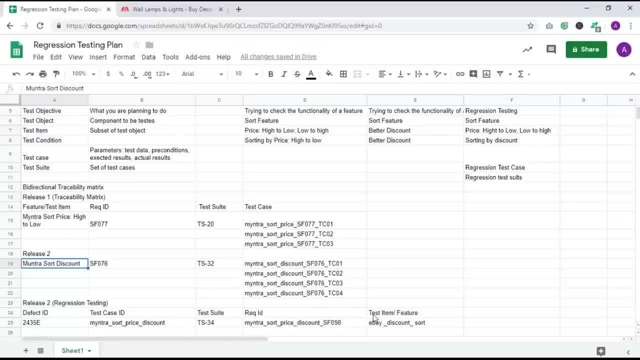 So from the defect we're tracing back and coming back to a feature which were testing on. you got my point right here We started with our feature or item and then we traced back to test case. But here we started with the defect and then we came back to a feature, so defect. 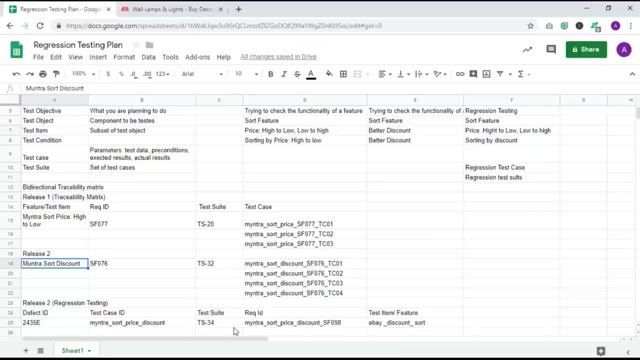 which is the test case ID that we're checking on the suit, which test case belongs to and was the requirement of the test case, and then the item on which it's being tested. So this is bi-directional traceability matrix. Well, this is just a small part. 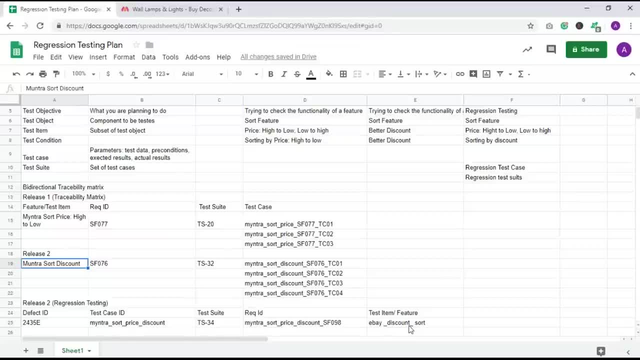 of you can say a million small part of what you can perform in testing. the very simple example like that, you can perform multiple traceability mattresses, multiple releases and in one release only, multiple tests. So basically, what I'm trying to say here is that this point, this item, is dependent on other features. 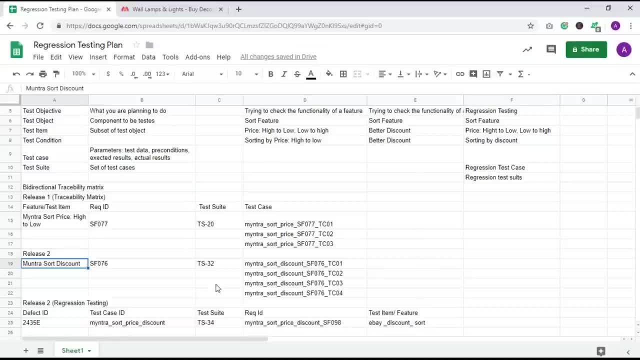 like, the discount option is dependent on high to low and low to high. So whenever you're trying to make any changes to discount option, your high to low or low to high options are not working, or either they're working or not working. from that You can tell these two things or the two items are related. 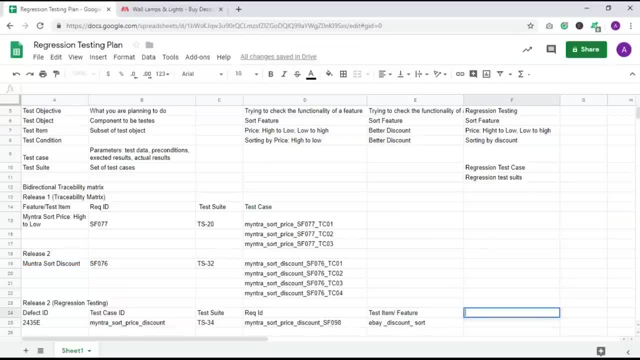 to each other or dependent on each other. for that you have, or you can add, another parameter called dependent features. So what are the features which are dependent on our discount, its price High to low, similarly mantra sort price, and what are the test cases which are dependent? 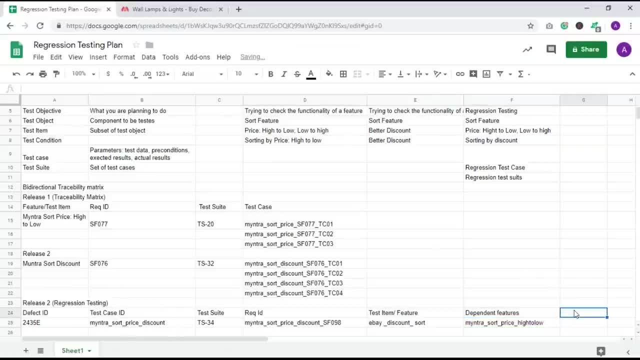 on this defect ID or the test case that also you can represent here. Maybe this test case is not dependent on it and this test case is dependent, So what you can do is going to copy it and paste it here. So this is the one test case. 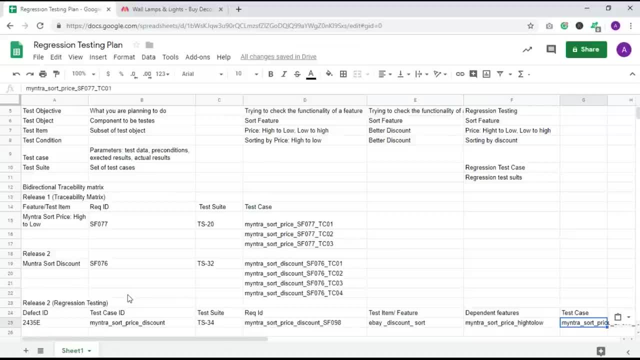 which is dependent on the discounting. So that's how you write a traceability matrix. I hope the thing is clear for you guys. So we just started with the basing testing. as in one feature, everything worked well. We have certain test cases and the test suit and proper. 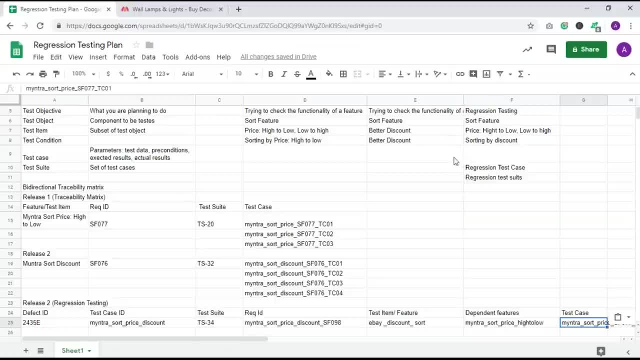 then you have another feature, which is better discount. based on that, you perform test. It's working well. Now you try to arrange everything from high to low and then apply discount. then you're getting in defect. based on that defect, We create a new one. 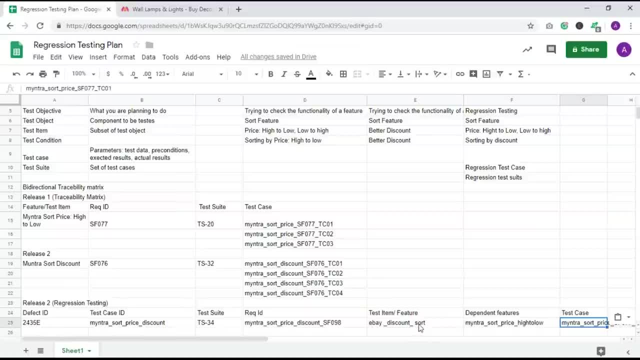 and we created a traceability matrix. We traced it back to our feature, which is sort, and the sort feature is our other features are dependent or interrelated to each other, So that's how they're affecting each other. So for that we need to perform testing from the beginning again. 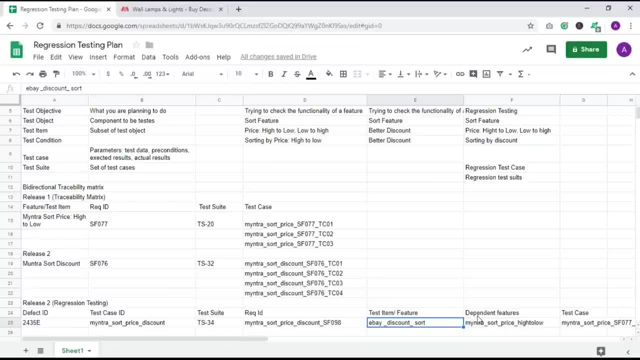 check out what are the errors and find out the defects and fix them. So that's what regression testing is all about, guys. So any changes that are added or made- it could be adding new feature, updating the existing feature- You should check if it's affecting the already existing functionality. 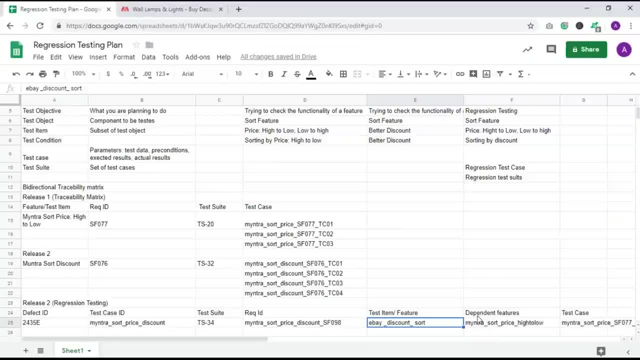 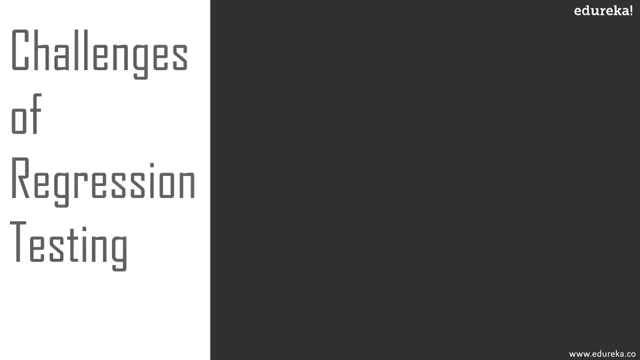 of your application or software. that's what regression testing is all about. So that's all with the demo. Let's move on to the next part. So regression testing is easy to define and understand, but baffling when it comes to performing regression testing of a software product. one reason is the dynamic nature. 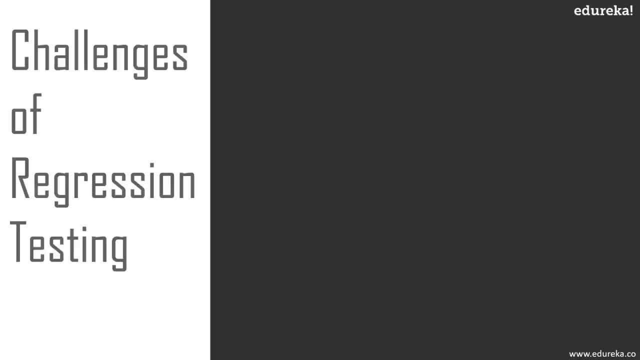 of software product. It keeps changing. You need to understand the challenges well before you can craft a counter strategy for these challenges. So let's have a look at common challenges of regression testing. So the first thing: regression testing is often considered as a drain of resources and manpower. to test again. 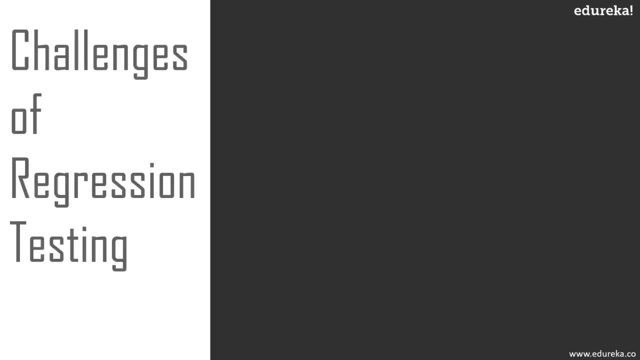 and again something which has already been developed, tested and deployed at early stages. So when testers are told to perform regression testing, that tempted to perform exhaustive testing of the software product quality assurance manager needs to make sure, or he needs to devise an intelligent methodology for regression testing to assure that every required test case. 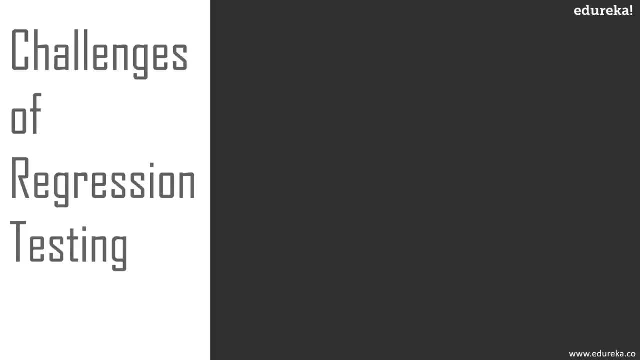 has been executed within the limited span of time and the amount of money that he's assigned with. So, basically, the first challenge that you'll encounter is it's time-consuming and expensive. So, as a Q analyst or manager, you need to devise an intelligent methodology. 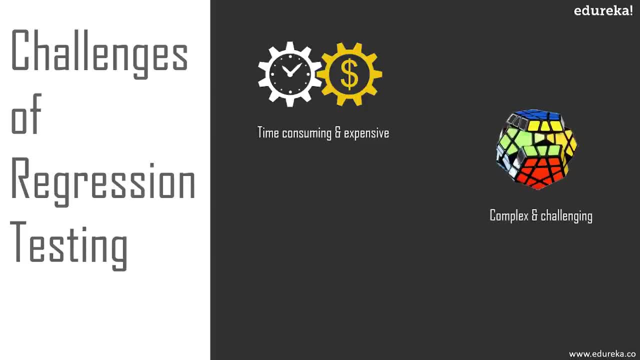 for regression testing. next test. It's complex and challenging as new features and changes are implemented in software product. more test cases are added to regression test suit as the product functionalities expand, testers are overwhelmed by the regression test cases and the fall victim to lose track of test cases. 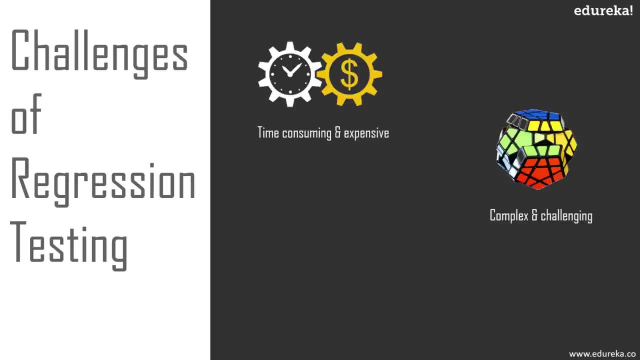 and when they lose track of the test cases, they overlook the important test cases as well, right, So regression testing is a complex process. This can be prevented by regularly monitoring the regression test suit and deleting the obsolete test cases. It is also important to avoid any duplication of test cases. 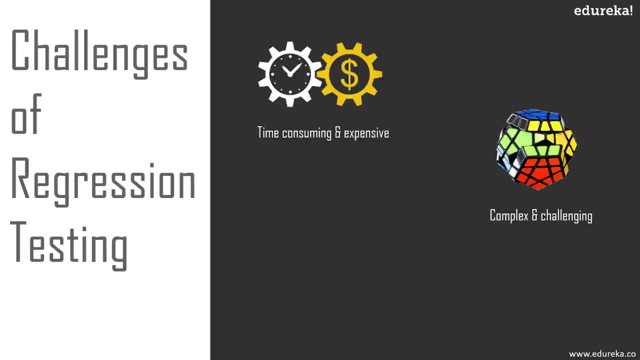 as they lack, to unnecessary effort and frustration for testers. Lastly, it's the communicating business value, and regression testing is usually tough regression testing, as you know, and just existing product features are still in working order. communicating the value of regression testing to non-technical leaders of your company within your business. 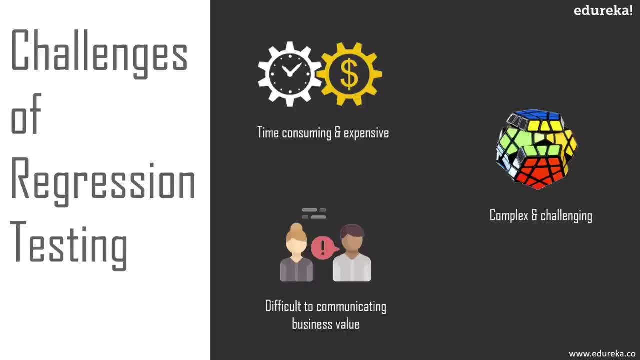 is a very difficult task. Executors most of the time want to see the product move forward. making a considerable investment in regression testing to ensure existing functionality is working can be a hard task. So these are certain challenges that you'll come across when you're performing regression testing. 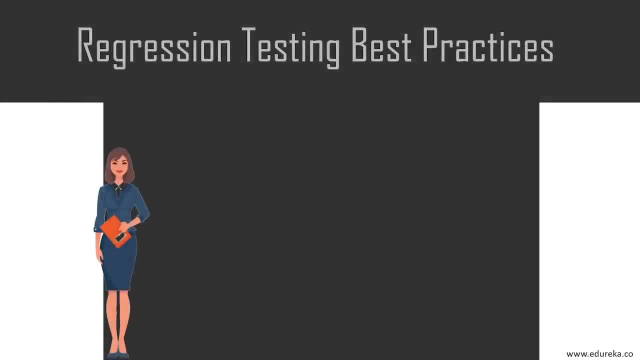 So, regardless of the method of implementation that we discussed earlier, that is, retest, all select and prioritization, There are a handful of general best practices that you can follow while implementing regression testing. that way, you can overcome the challenges that we discussed earlier. So the first thing is you need to maintain a schedule. choose. 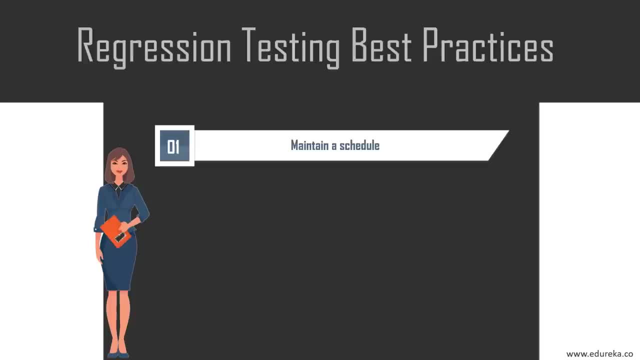 a schedule of testing you can maintain throughout the software development lifecycle, So testing is never placed on back burner. Secondly, use a test management tool in order to properly keep track of all the tests that are being performed- a regular basis- and have the records of their performance over time. 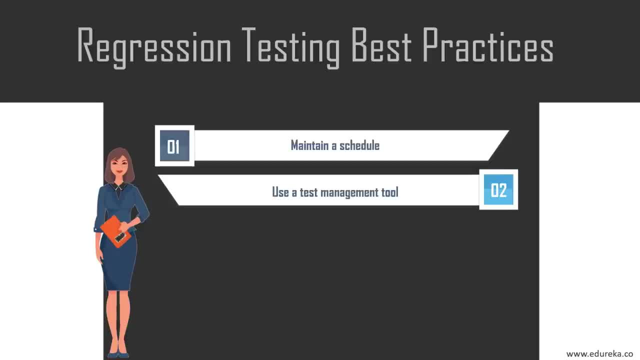 It's better to use a simple kind of test management tool that does all the tasks for you, instead of you spending long amount of time and efforts on keeping track of all these test cases. You can break down and categorize your test. tests are often considered to be easy to understand. evaluate. 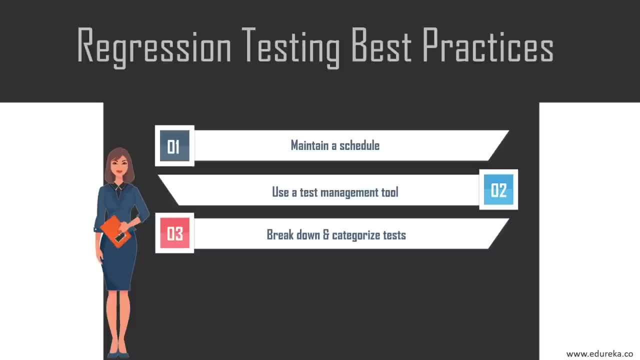 if they are broken down into smaller pieces. It's not just with testing anyway, right, If the thing is huge and complex, it's difficult to understand, but if it's broken down into pieces and then you try to understand, it's easy. So try to refactor your test cases as often as necessary. 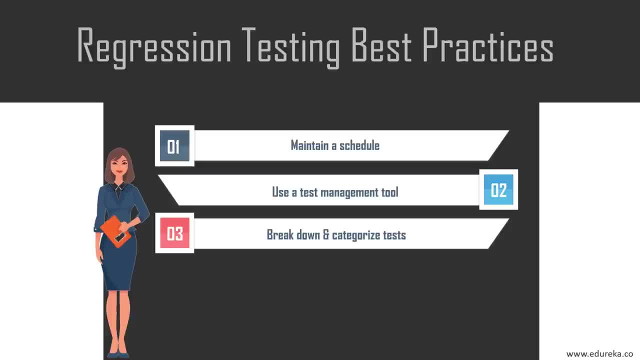 then categorize them such that the categories of smaller tests can be prioritized over the others. So this makes sorting and execution much easier and future for you. You can do this. you can also consider customer risk, not also. you must and should consider customer risk. basically, the product. 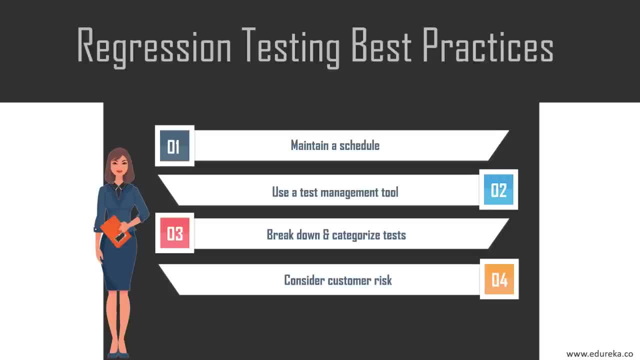 is made for customer right. So when developing and prioritizing regression test, keep track about considering the effects the test cases will have on the customer or the business as a whole. So try to design such test cases that they cover as many test cases as possible. 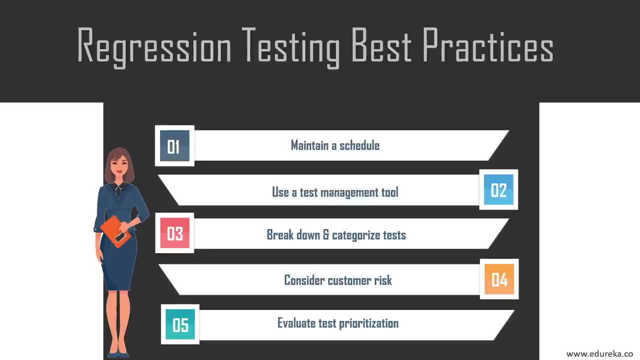 and lastly, evaluate test prioritization. So when using any form of prioritization to order your regression test, try to find a sensible way to order them, such way You know what you're actually doing. don't mess it up So well. these are certain things that you can follow.